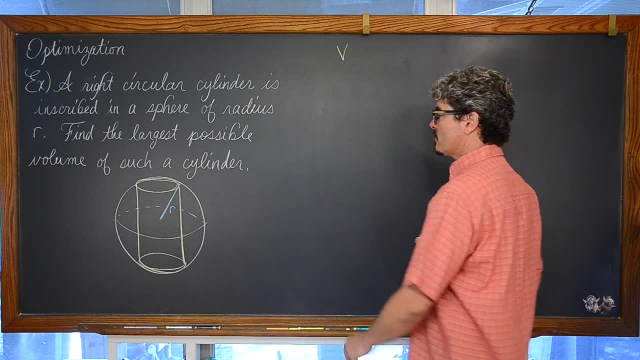 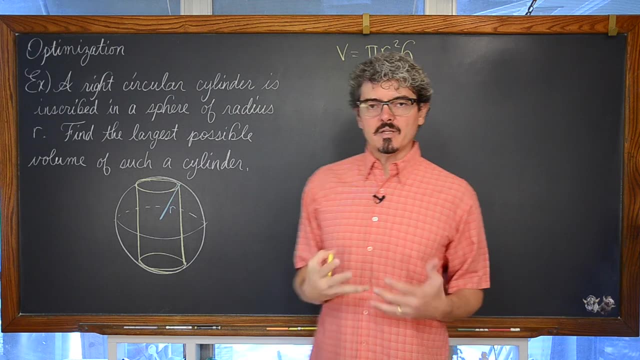 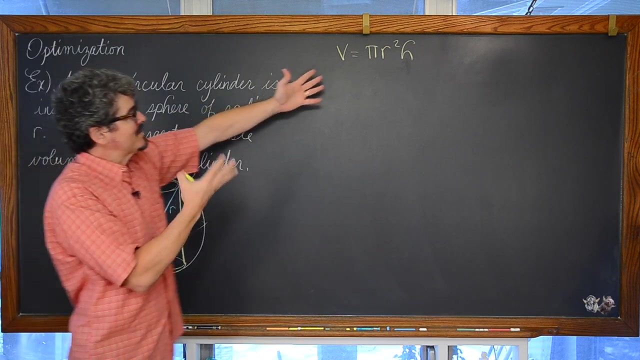 So the volume of a right circular cylinder, of course, is area of the base. So volume is equal to pi r squared times the height. Just kind of pulling that formula out of geometry, But that isit is obviously the formula of a right circular cylinder, but it is going. 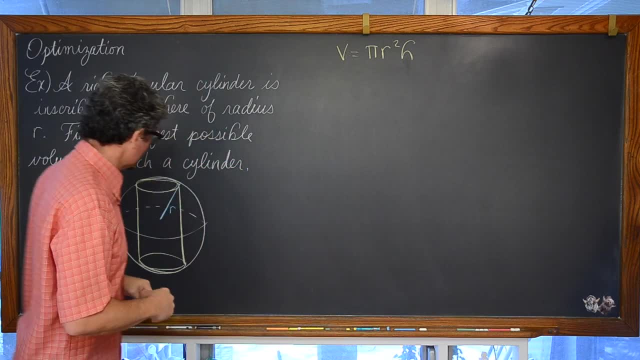 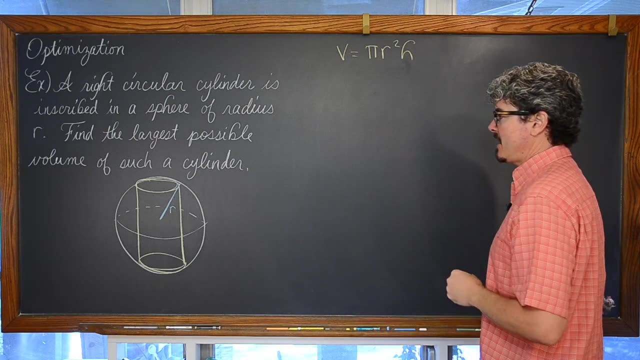 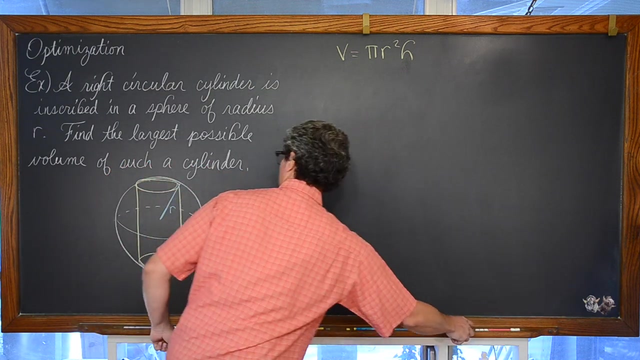 to be a little bit confusing when we see this r here for the volume of a cylinder and the r which is the radius of the sphere, because they are not the same. This islet's see here: what color can I usegreen maybe. Hopefully that shows up differently on the camera, Or. 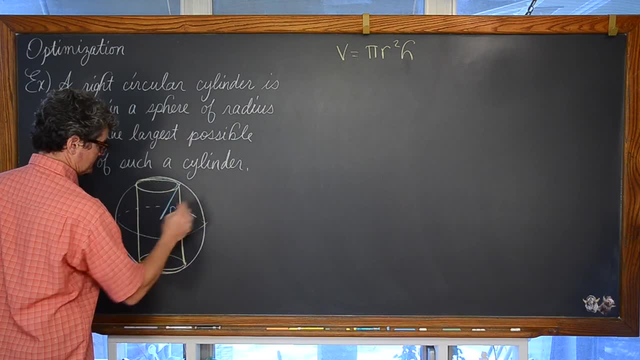 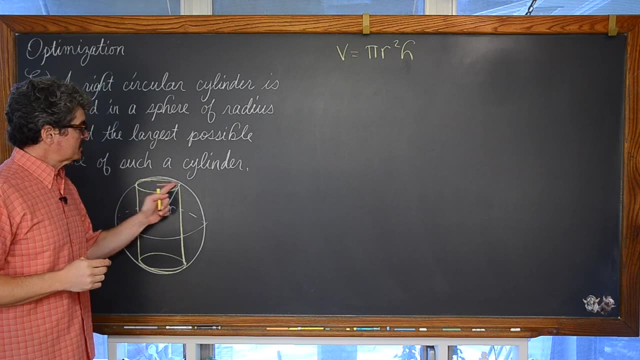 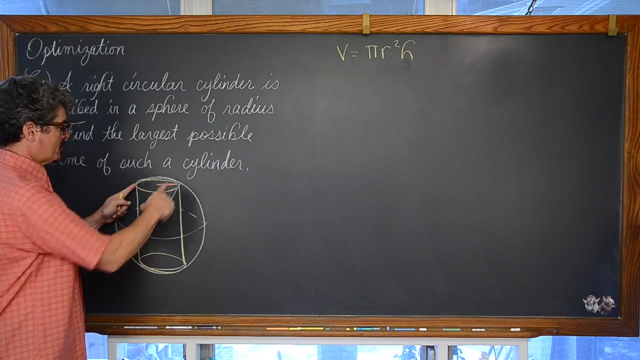 red. There we go, Let's use red. It is the r thator. at least that is the radius of the right circular cylinder. I am going to call it a cylinder And that radius is variable. So whether I draw the top and 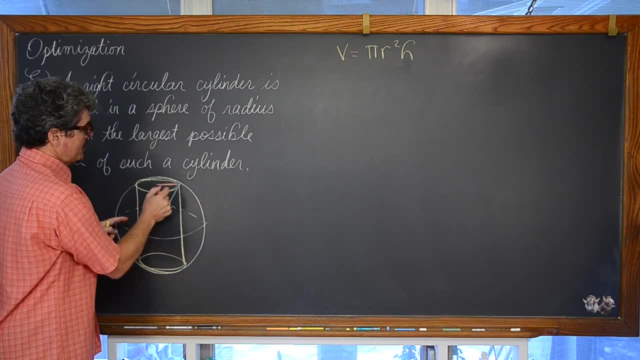 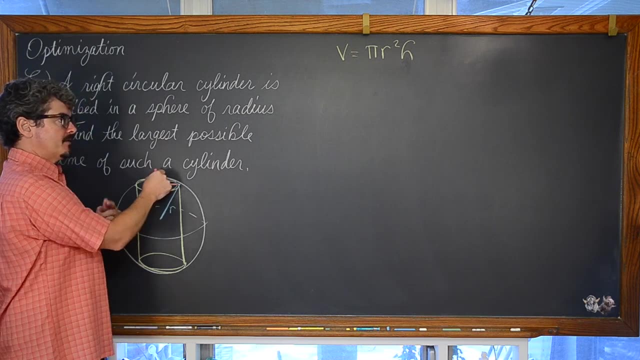 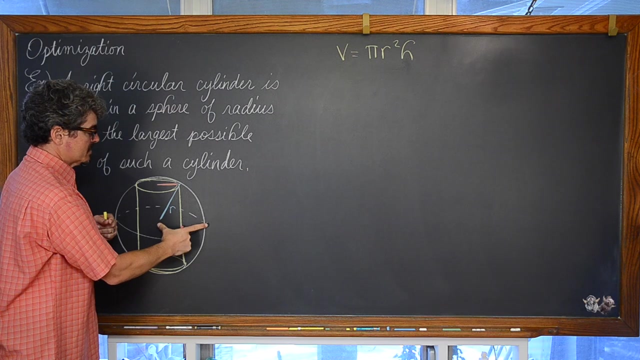 the bottom of the cylinder, here or here or here, that horizontal distance is going to, of course, change from basically potentially down to a theoretical radius of zero, Down to, but not including, zero, And then that horizontal distance can go up to as much as the radius of the circle I. 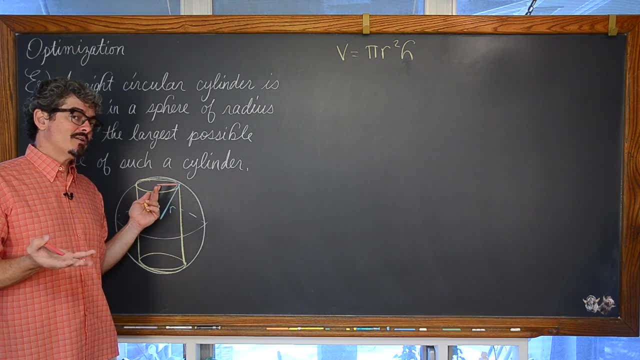 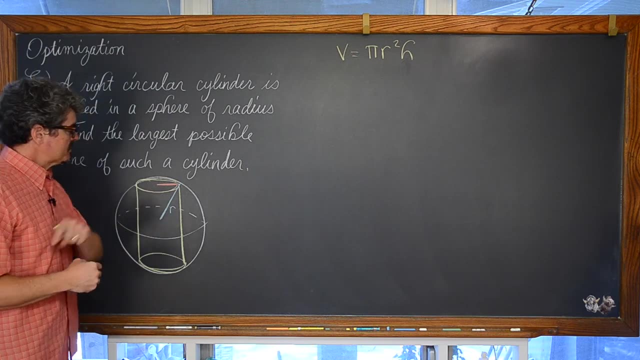 guess you could actually have an x value- which is what we are going to call it- of zero, But then you are not actually going to have a cylinder that has any volume, Same as if x is equal to r. So we are going to call this and label this with the variable of x. So 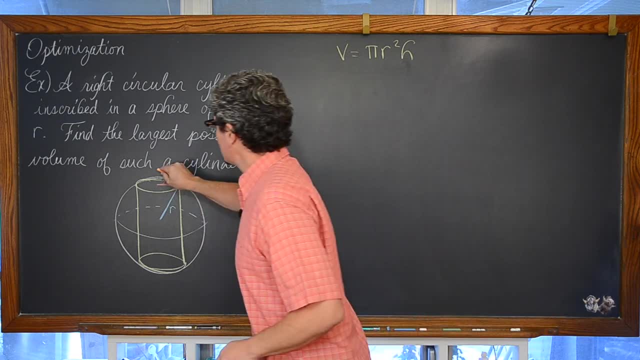 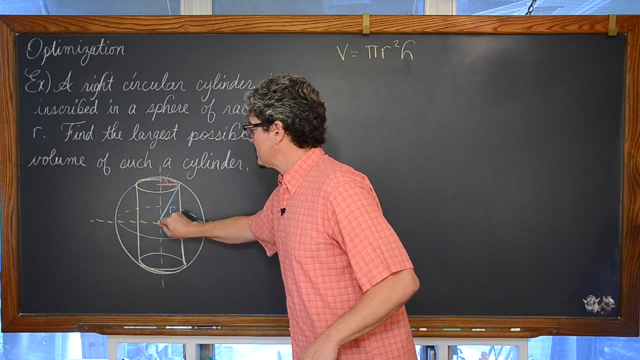 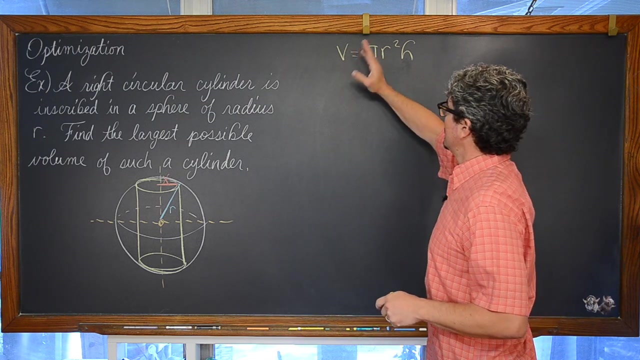 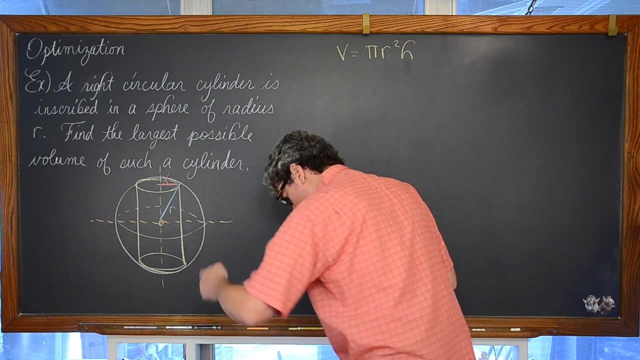 kind of think about us having an x- y axis here, where the center of the sphere is the origin. Okay so, volume of a cylinder pi r squared times h. we are going to call r. Label that with the variable of: oh no, brand new piece. 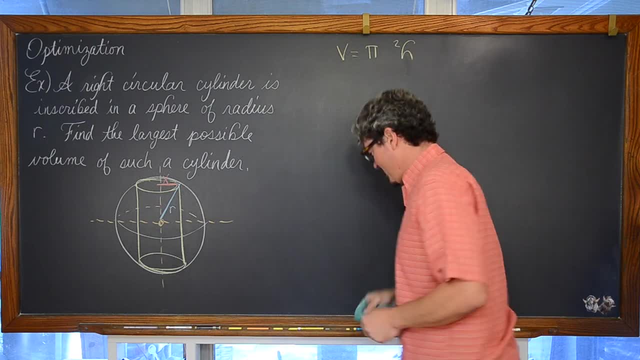 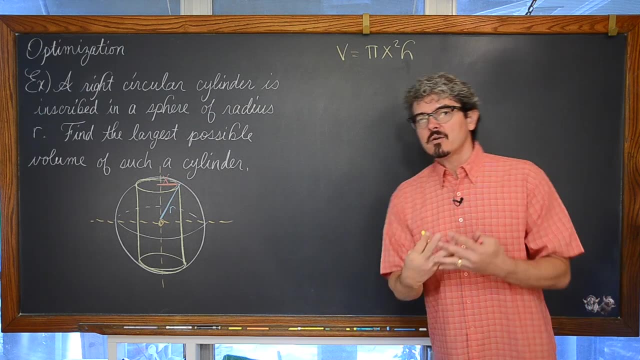 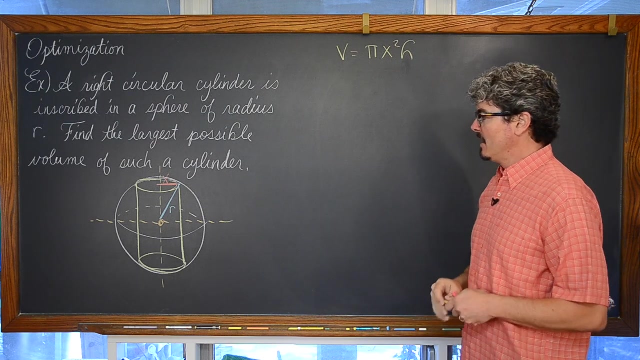 of chalk down and now two pieces of chalk. We are going to call that x. And now we need to figure out a better label or identifier for the height of the cylinder in context of this problem. Well, if I have the origin in the center of the sphere, then our vertical 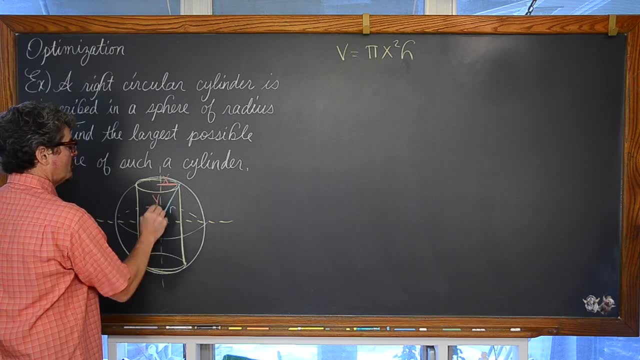 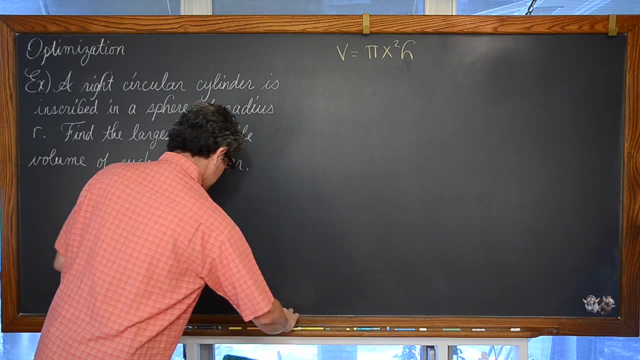 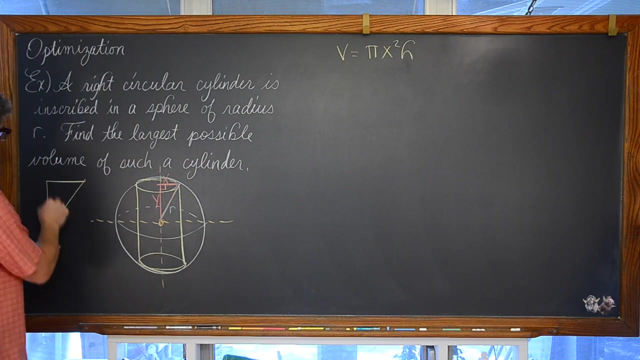 distance is going to be labeled with y, and we are really breaking down and working with this little right triangle right here. Okay, so, pulling that out to the side, we have a triangle, A right triangle, whose hypotenuse is going to be the radius of that sphere. We have a 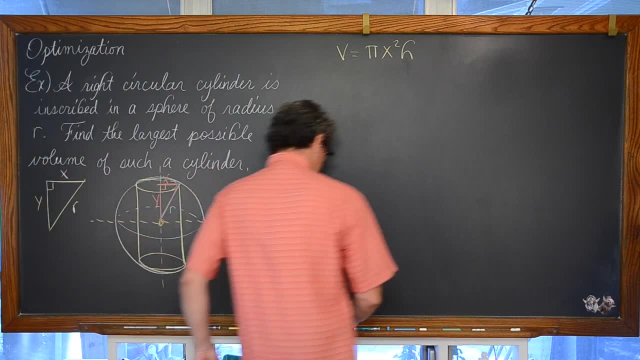 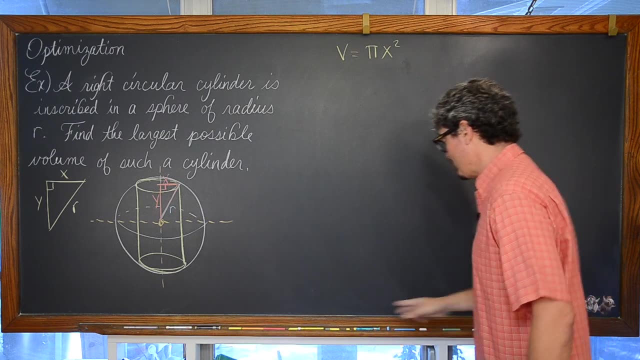 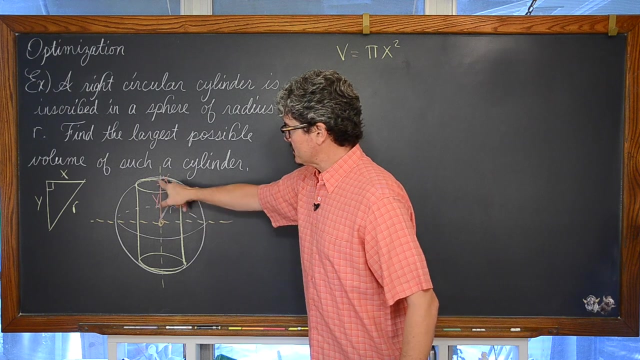 horizontal distance of x and a vertical distance of y. Okay, so converting y into some more usable identifier for this particular function or this situation, this problem: the height of this cylinder is not equal to y. The height of this cylinder is equal to y times 2 because 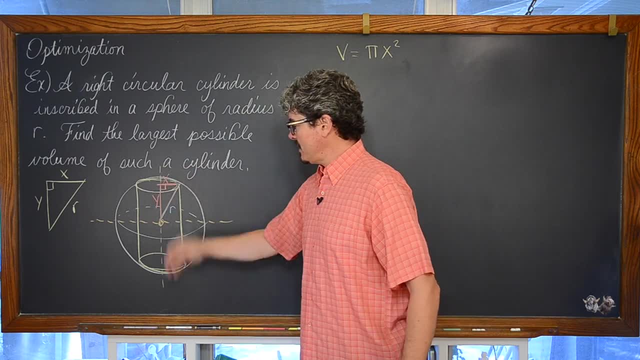 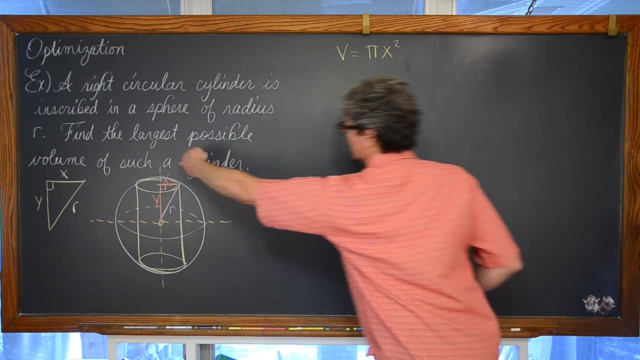 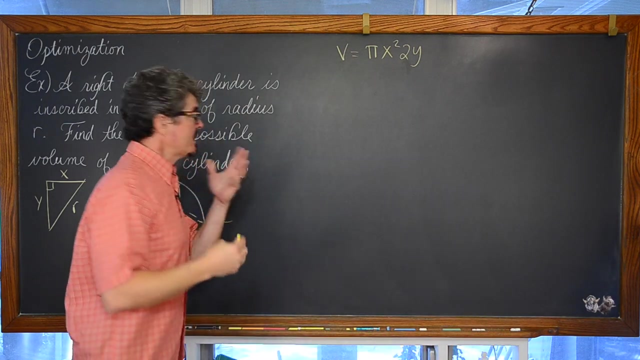 we have a lot of symmetry And since the size of both bases- the top and the bottom of the cylinder- are the same, that is going to be doubled. So the height of this cylinder is equal to 2y. Okay well. 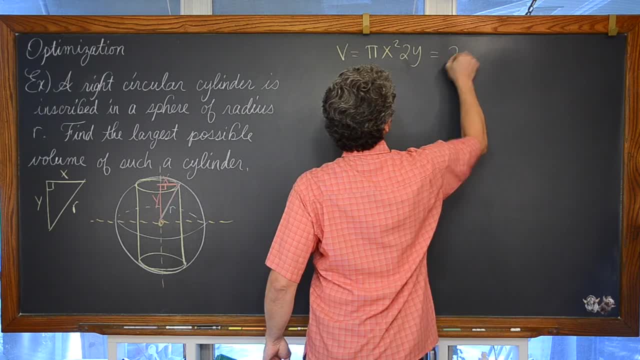 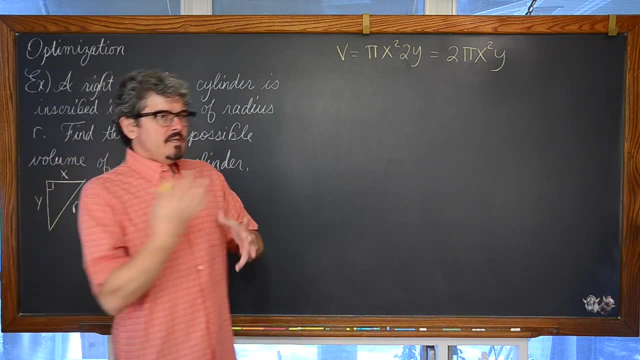 that is great. So we are looking at basically 2pi x squared times y. But here is where we need to bring in that fixed value. Which? what is that fixed value? Well, that is the fixed value of x squared times y. Okay, so we are looking at basically 2pi x squared. 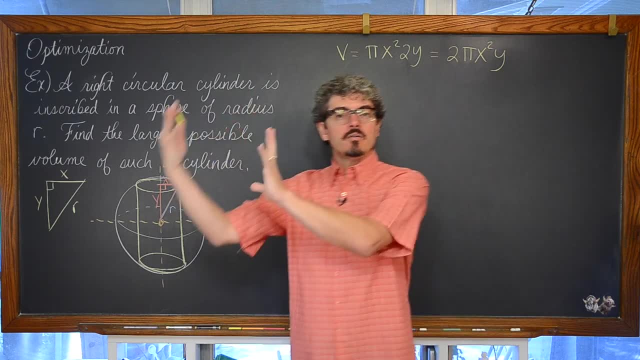 times y. But here is where we need to bring in that fixed value which we are looking at basically 2pi x squared times y. So if a question was about variable volume with a fixed surface area, we would have to do some kind of substitution to bring information. 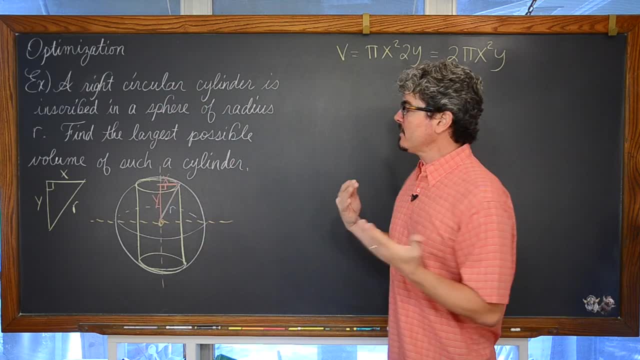 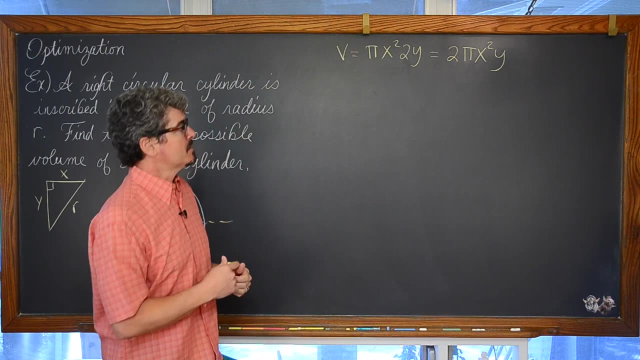 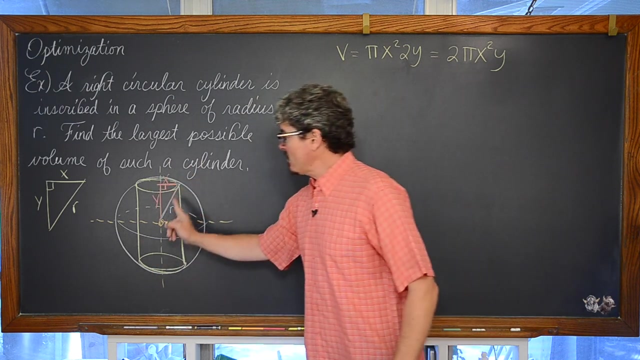 about that fixed surface area into the volume. Well, the only thing fixed here is that information of r. We need to not just find the volume of any right circular cylinder, we want the volume of a cylinder that is inscribed in this sphere with a radius of r. We somehow 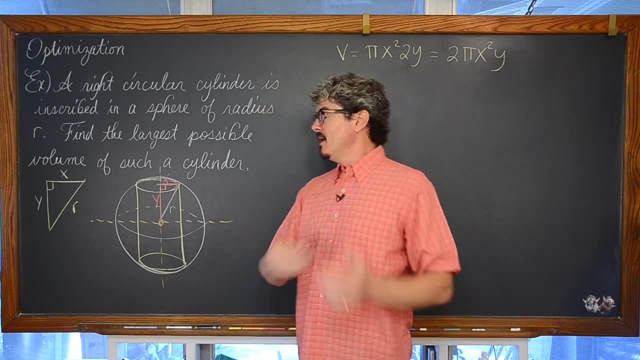 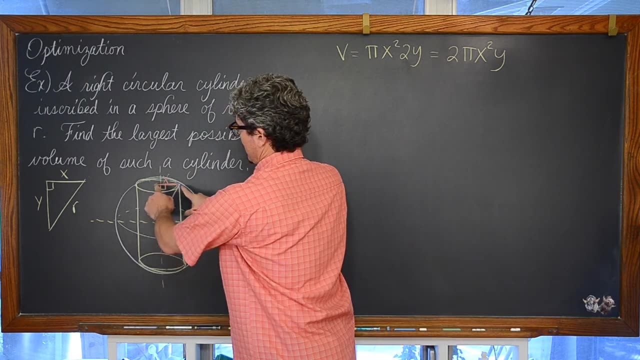 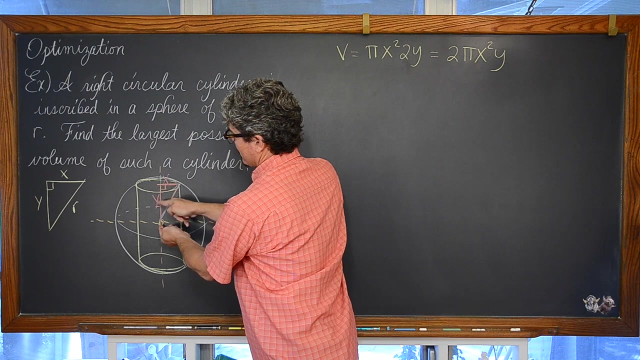 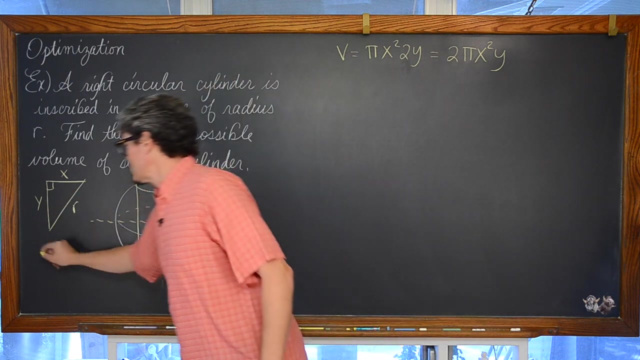 need to bring in that constant, though it is unknown constant value of r. Again, as we draw different versions of the cylinder, we can have different horizontal distances it takes to get to the edge of the sphere. Of course that is going to correspond with different heights of that cylinder. Well, it is a right triangle, So 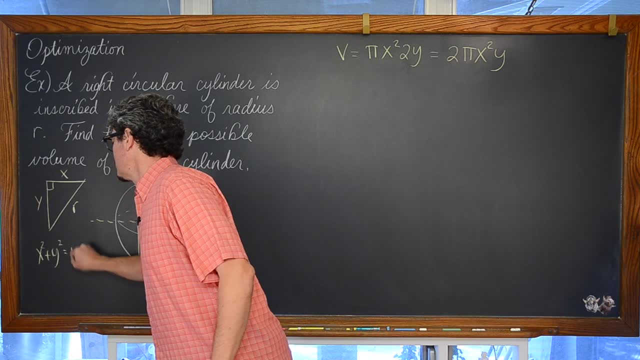 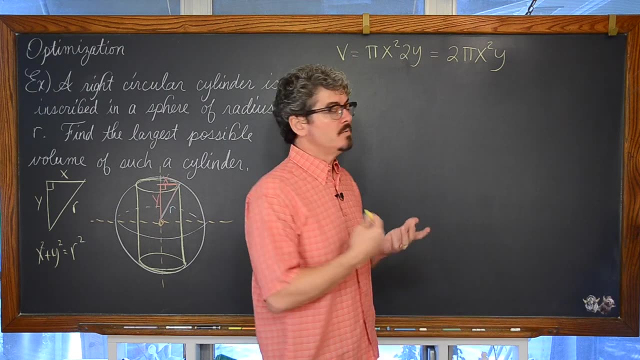 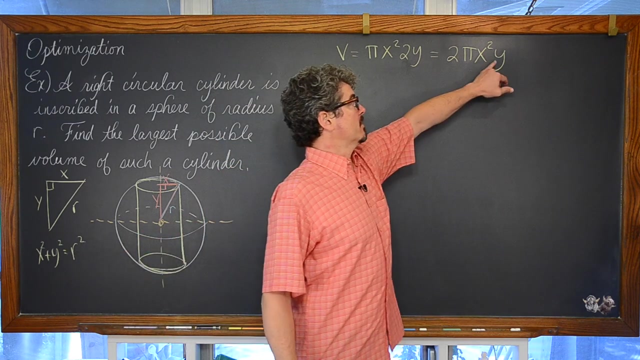 we have x squared plus y squared is equal to r squared. What is going to be easier to get out? Are we going to bring the fixed, unknown value of r into this equation through the variable of y or through the variable of x? Well, why would I want to solve for y and 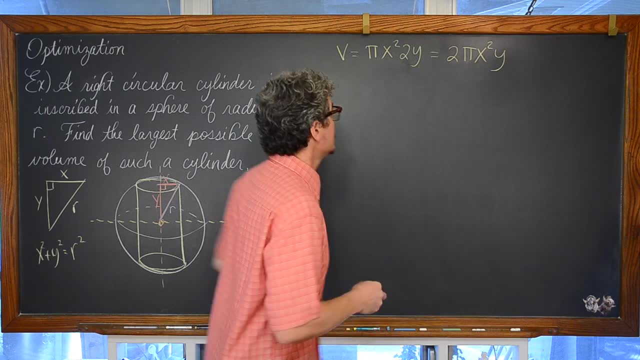 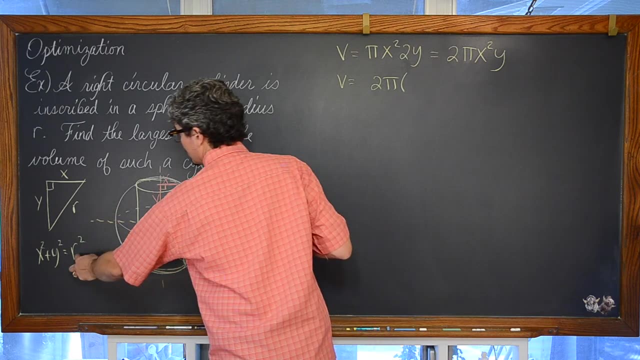 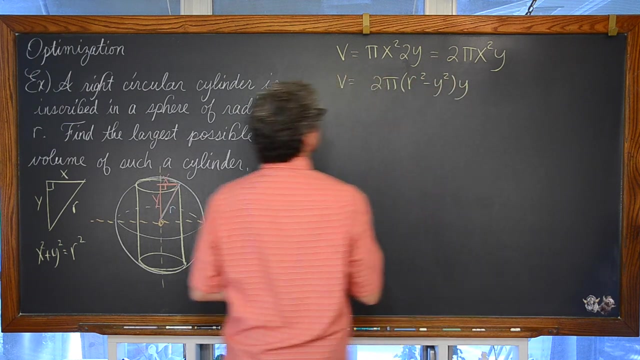 have square roots when I basically have a nice clean x squared here. So we have that volume is equal to 2pi x squared, Which is going to be, of course, equal to what R squared minus y squared times y, And now we have volume. in terms of what Is the volume? 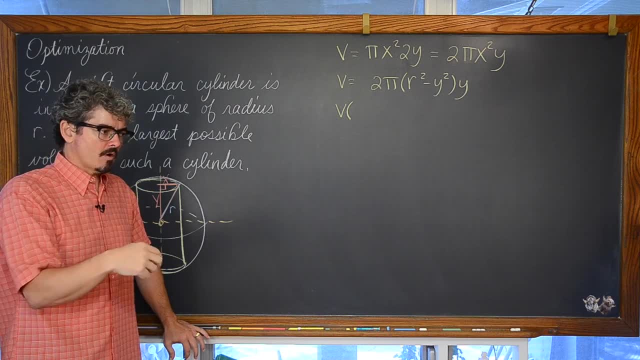 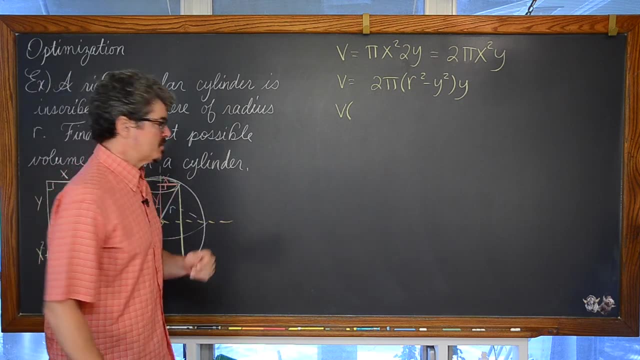 in terms of y or is the volume in terms of r? What would be more interesting, The volume of this cylinder is going to change. well, not based based. well, it is sort of based on the radius. Okay, things are changing. 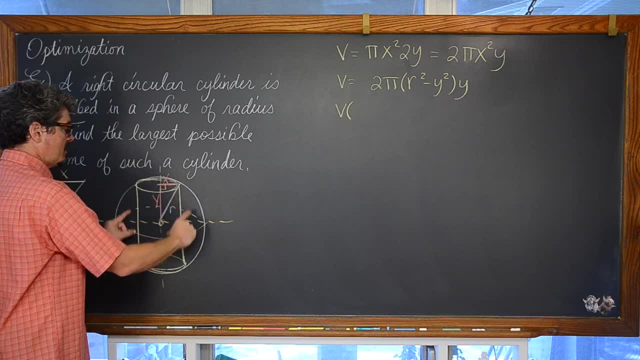 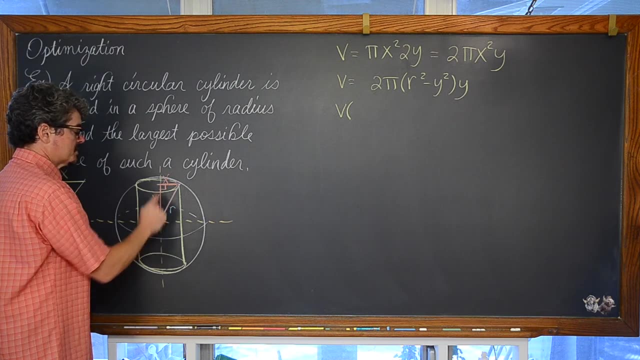 Actesparency in the fourth quarter times. y always weights the curve, It is not done much of the cylinder. but more importantly, we're changing the shape of this cylinder inside the sphere based on that vertical distance of Y, which is the distance away from the origin. so we need this. this is basically volume in terms. 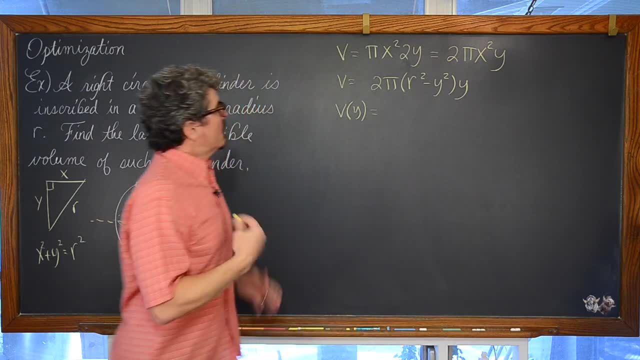 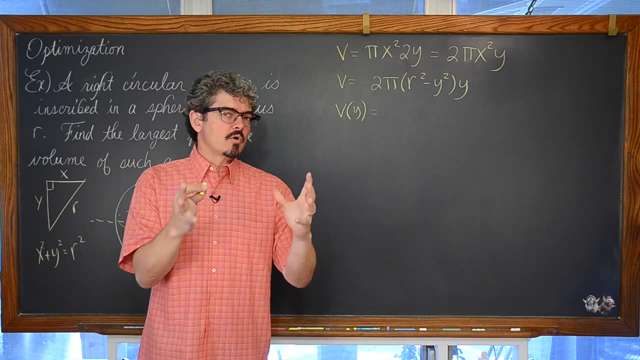 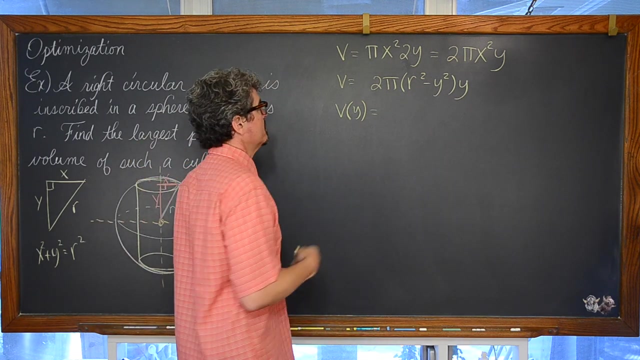 of Y, and I'm also going to go ahead and distribute all this together, because what's the next step after setting up your primary function, with optimization problems, after you bring in that's, that information about the from the secondary function or that fixed value, you need to optimize it, you need to set. 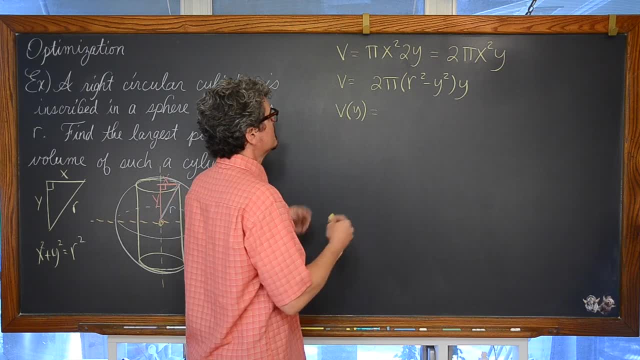 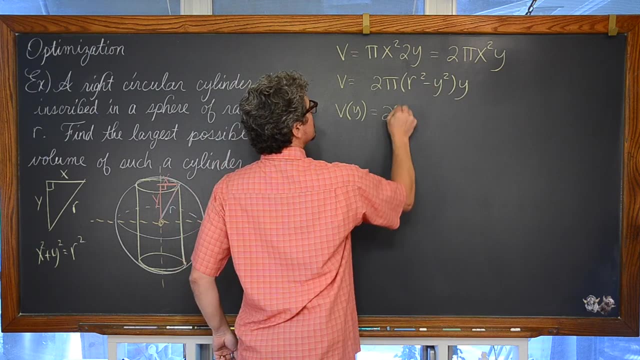 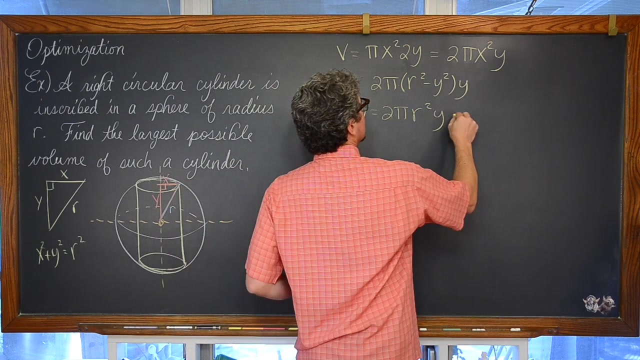 the set up the first and use the first and or second derivative test to find where that function is either at its maximum or minimum. so 2 pi Y times R squared, 2 pi R squared Y, and then 2 pi Y times negative Y squared is negative 2. 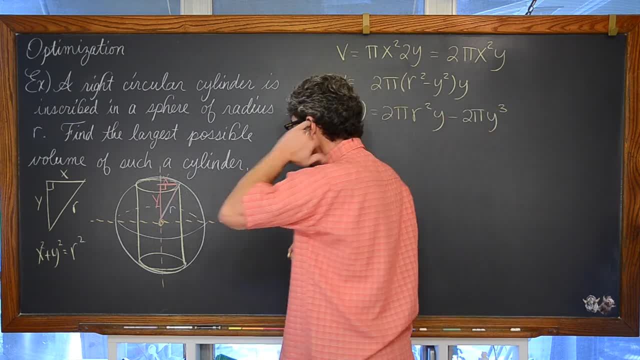 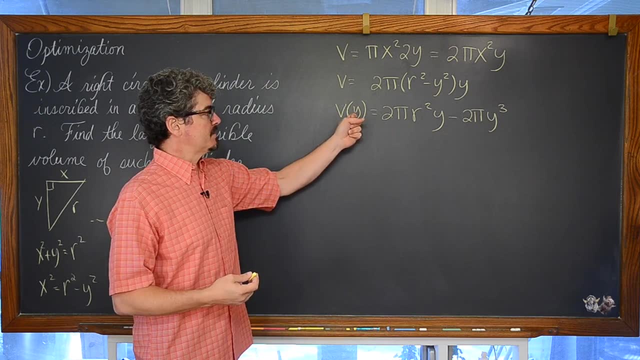 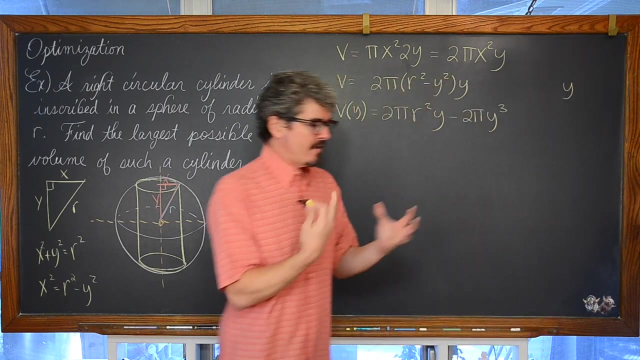 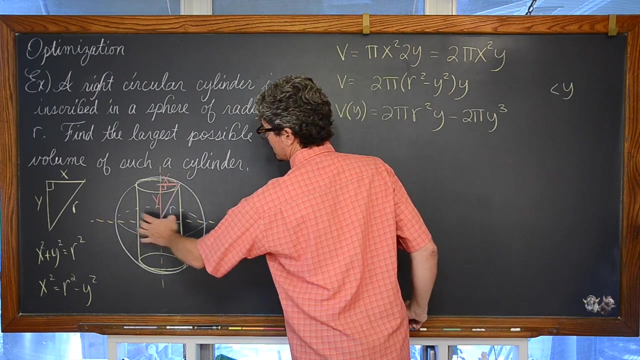 pi Y cubed. okay, now we need to run this through a you know find out where, for what function or what value, excuse me of y. oh, by the way, domain, what is? what kind of values can Y take on? well, Y can take on values from up to 0. where your cylinder, if Y is? 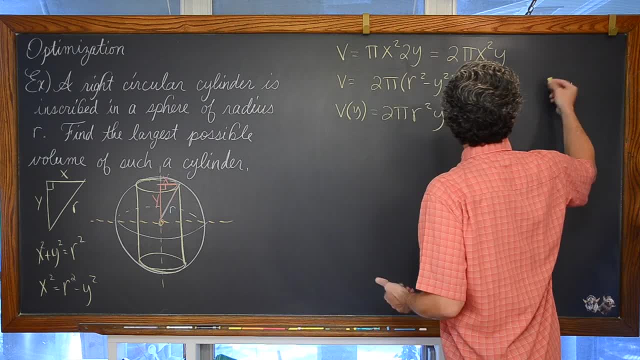 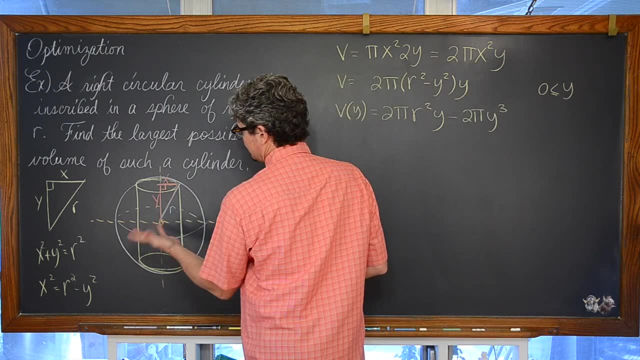 equal to 0. you can actually kind of argue that I'm going to say that Y is going to be greater than 0. you could argue it could technically be equal to 0. but if Y is equal to 0, well then you don't have a cylinder, you just have a. 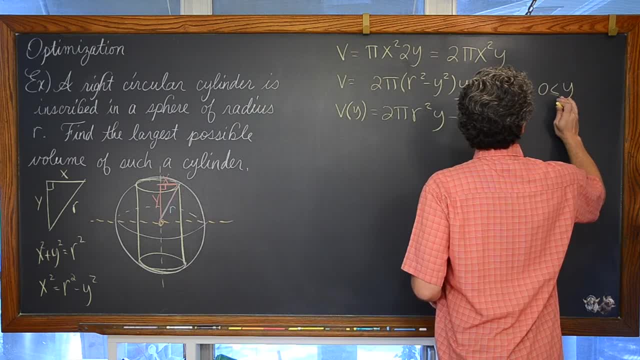 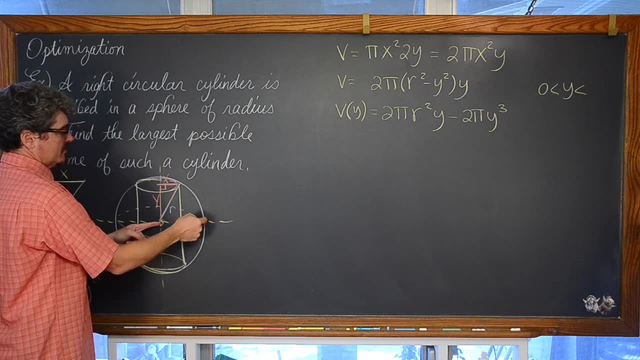 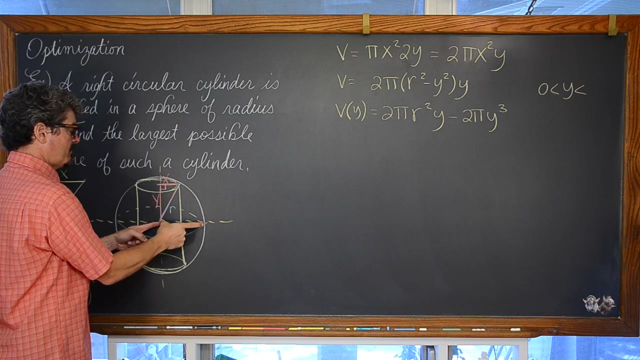 circle. so I'm gonna say the Y is greater can be values that are greater than 0 and less than what? as this radius of R kind of rotates up to pi over 2, that value of Y is going to go from a value of 0 up to a maximum value of R. 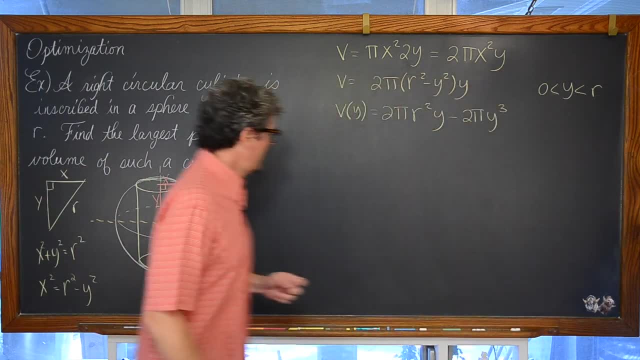 but I'm not going to say that Y can be equal to R, because, well, that's the value that we're going to be taking on in the next class. then, If y is equal to r, you don't have a cylinder, unless you want to say you have. 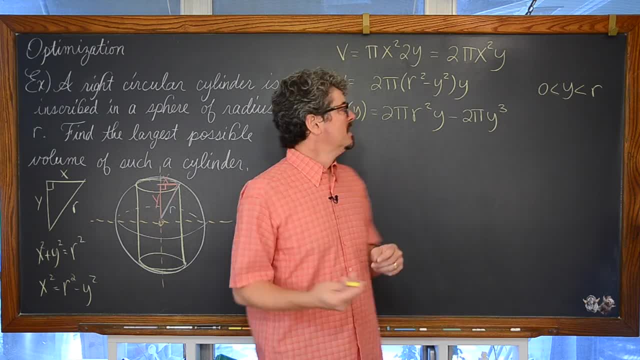 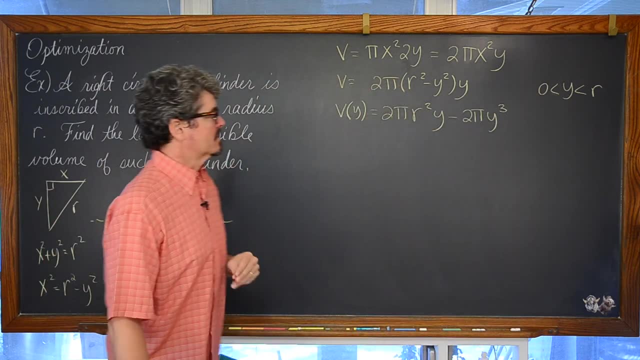 a cylinder with a radius of zero, but that's kind of just a line, And I don't know. maybe your teacher can argue that this is maybe you disagree with me that this should be a closed interval. I'm going to keep it as an open interval, though, If it is a closed interval. 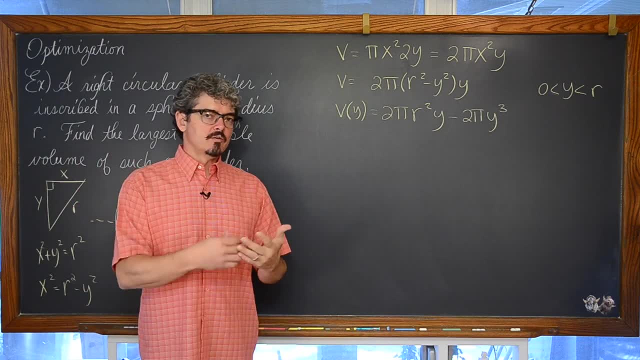 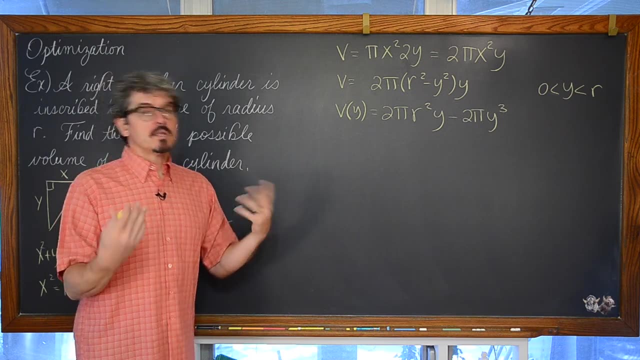 then you're just going to do sort of that extreme value test. So I'm going to work with the first and possibly second derivative test to find a sort of a- well, relative extrema. but if you only have one critical value on an interval, then that ends up being an absolute. 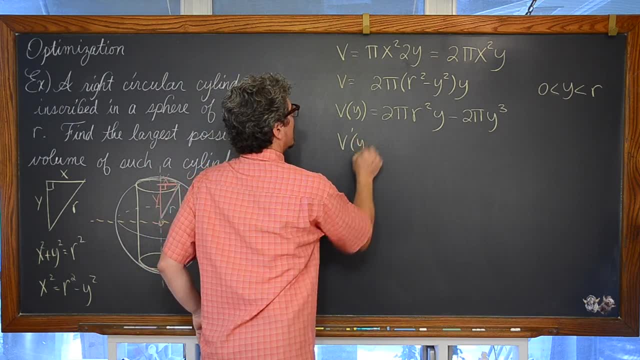 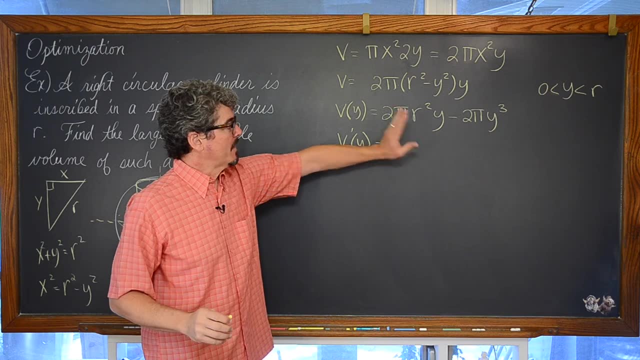 maximum. So anyway, v, prime of y. I don't know if you need me to review and verbalize all my thinking on this. You may be very advanced in calculus. hopefully not wasting your time As you take a derivative of this function. remember that while we do not know what the 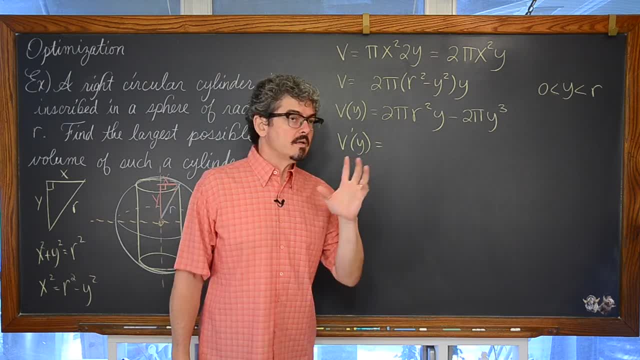 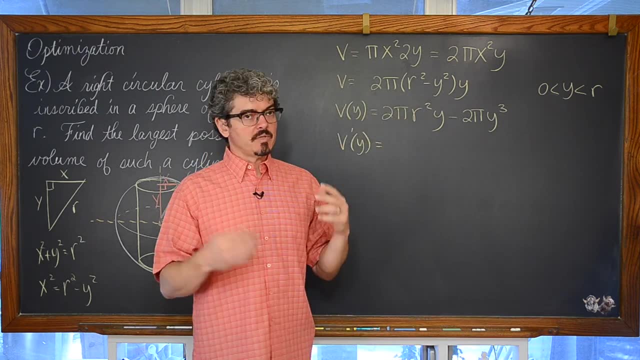 value of y is, and we do not know what the value of r is. r is being, for this problem, that fixed radius of the sphere. It's a constant. So you have a constant times, just simply y. Okay, And you're going to be taking a derivative with respect to y. So v prime of y is just 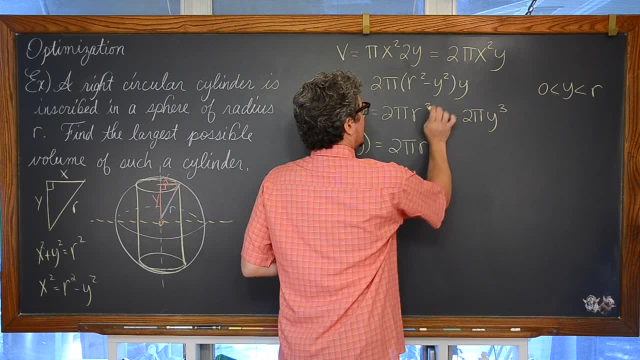 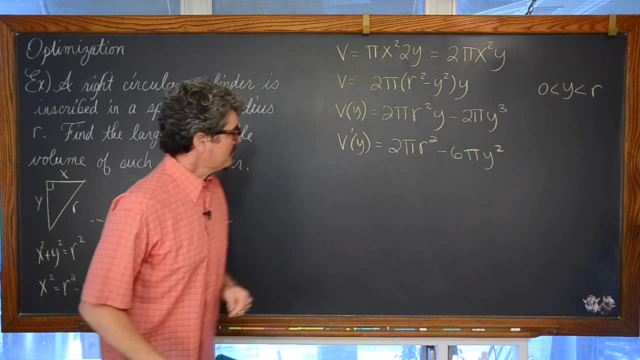 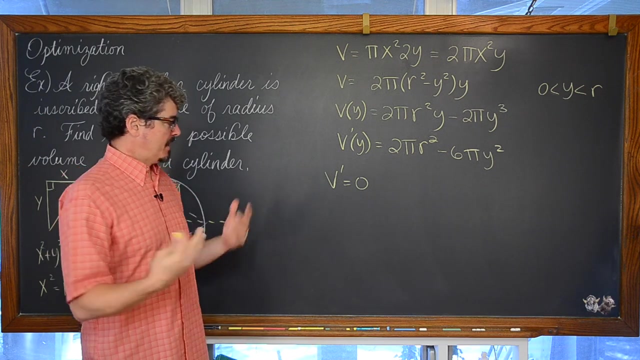 simply 2 pi r squared, And here, just using the power rule, 3 times negative, 2 is negative, 6 pi y squared, And we need to find out where v prime is equal to 0. And where it could potentially be undefined. but v prime is never going to be undefined, because this is really. 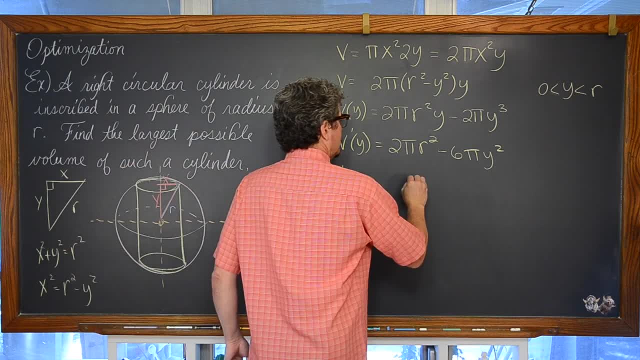 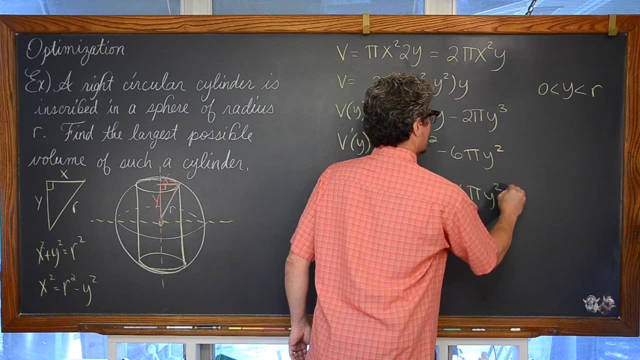 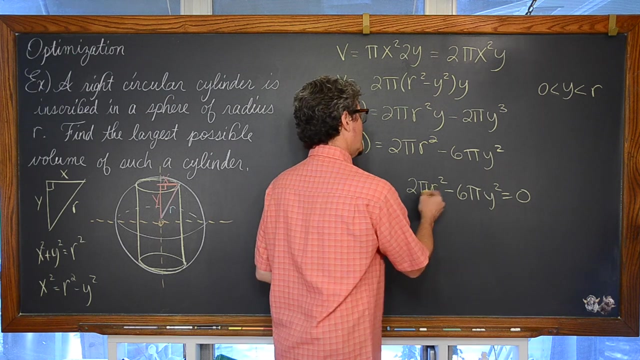 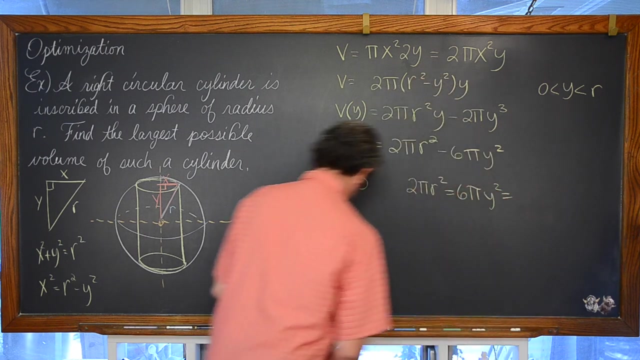 basically just a polynomial. So we have Setting the sequence. We have 2 pi r squared minus 6 pi y squared is equal to 0.. But of course we can just add both sides by 6 pi y squared, giving us that 2 pi r squared is equal to 6 pi y squared. 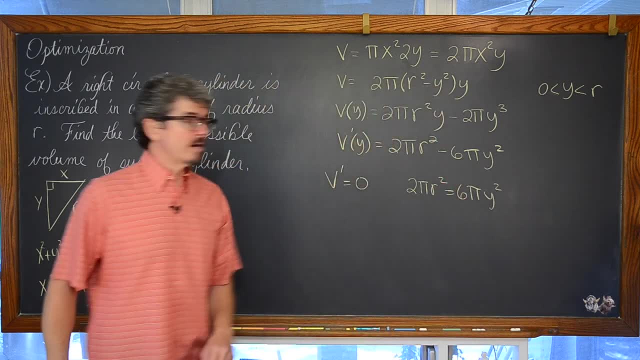 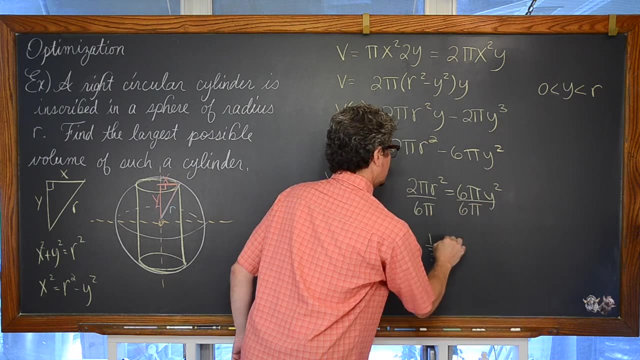 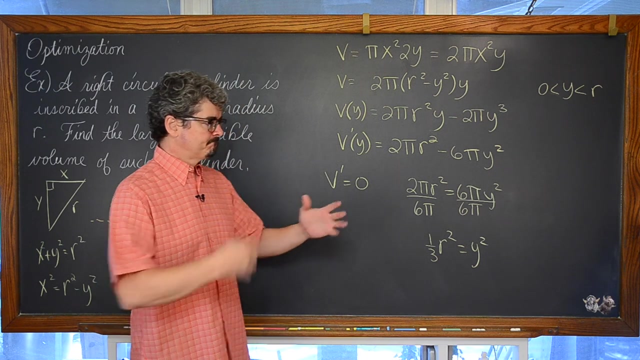 Dividing both sidesoops, Dividing both sides by 6 pi, we have, Okay, Okay, Okay, 1 third. r squared is equal to y squared, But I want to find the value of y that sets this derivative equal to 0, basically the critical value, Which means we're going to. 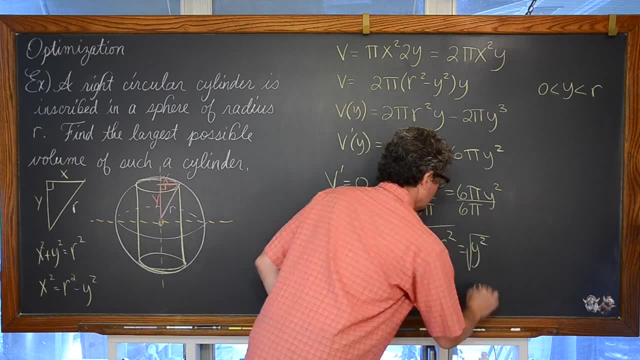 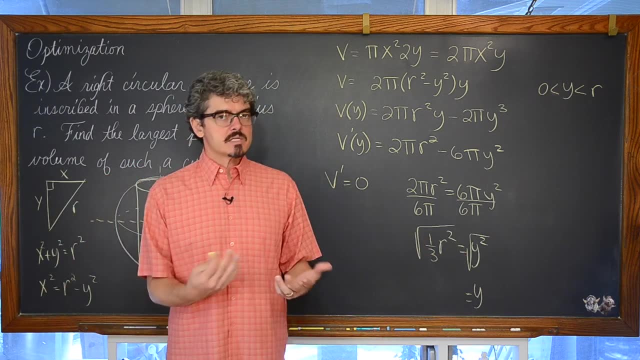 square root both sides And we have y is equal tonow. of course, when you introduce your own even root to both sides of a function, you have to account for both the positive and negative answer. But y can only be positive. 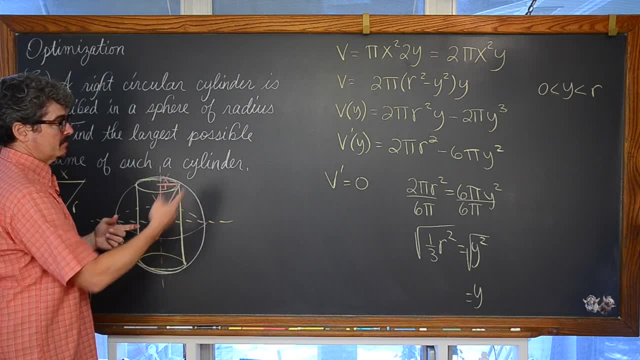 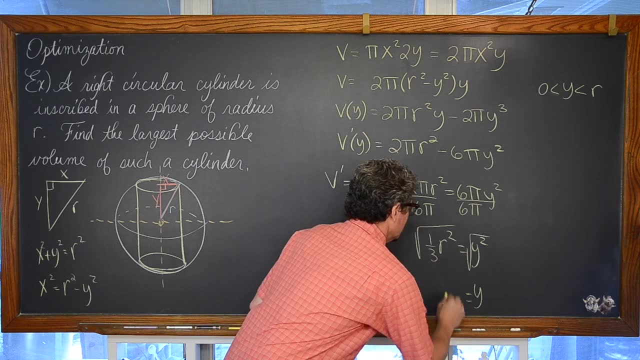 Okay, Since we're defining it as being between the values of 0 and y. So we have basically the square root of 3 over 3.. We have 1 over the square root of 3.. Rationalize that, of course. 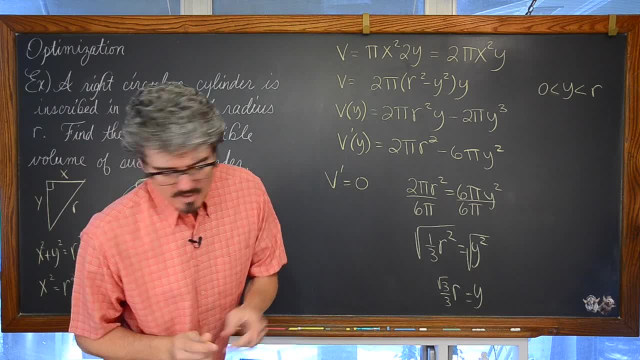 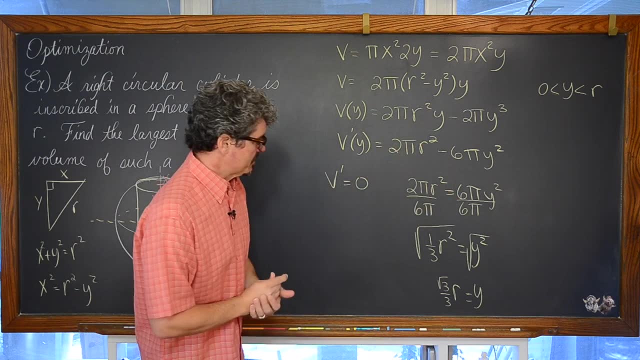 r. Now is thatlet me just check that. Okay, Now that's our critical value. That's where our first derivative is equal to 0.. If you reallyand I'm sure your teacher is going to make you actually do this, You know if this is a critical value that does. 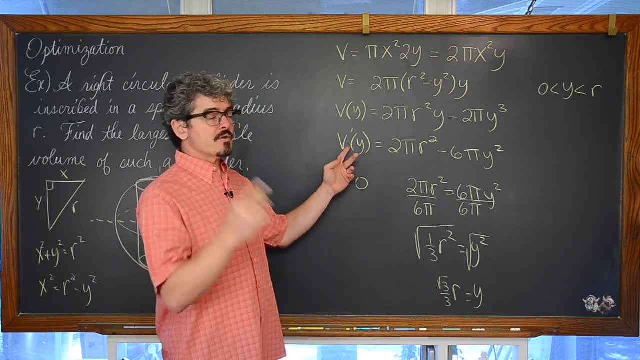 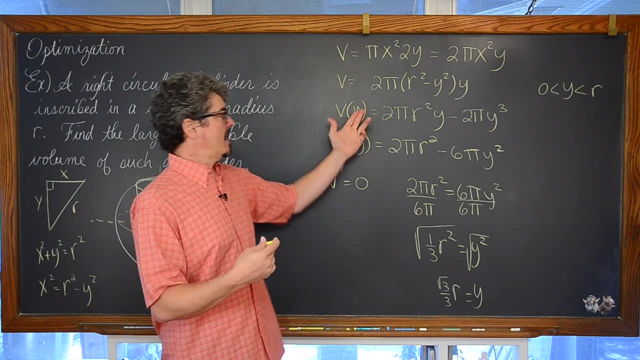 not mean automatically. you know, just hey, where the first derivative is equal to 0,, then this function of v is, you know, going to have an absolute maximum, Or even a relative maximum, Or minimum for that matter, Because this is just simply a critical value. You 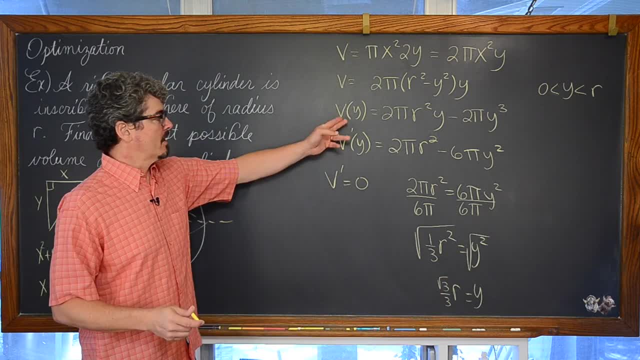 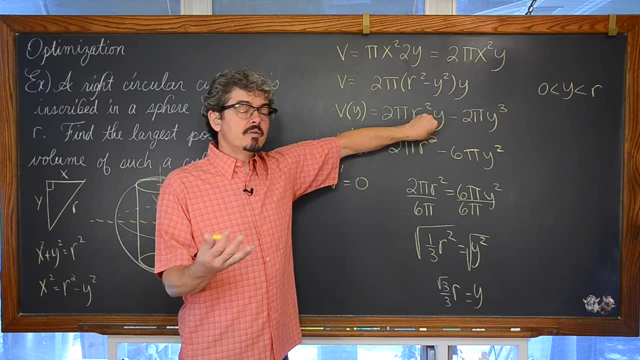 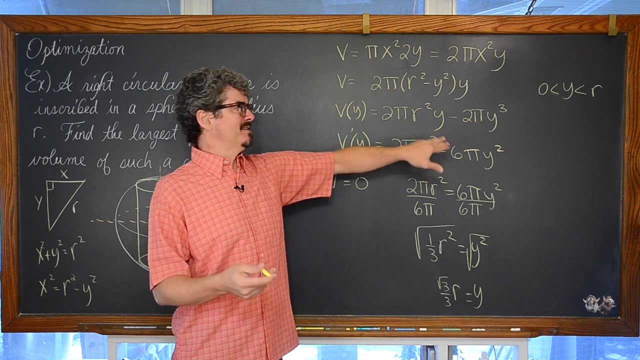 have to test whether or not this is a location where, well, this is a critical value for v prime. So does that mean that v of ydoes it have a maximum or minimum there? Well, maybe the first derivative doesn't change sign, Maybe this is just taking a rest and 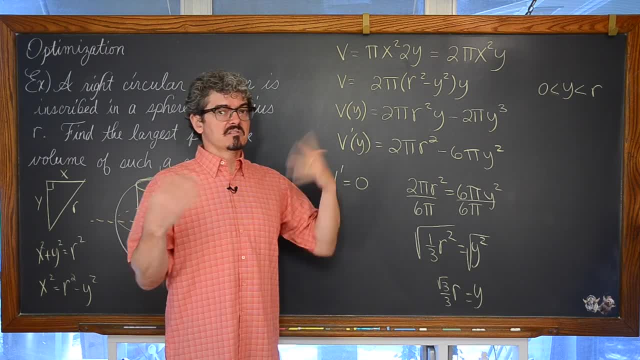 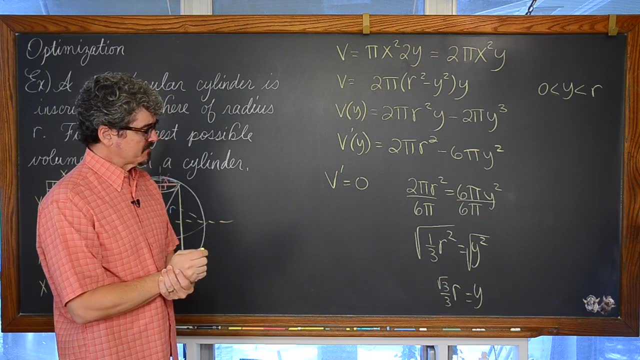 it's just, you know, for this critical value. this is just, I don't know, whatever The function is kind of maybe rising, leveling off and rising again. First or second derivative test. Now there's two things you can do. You can either look at your first derivative. 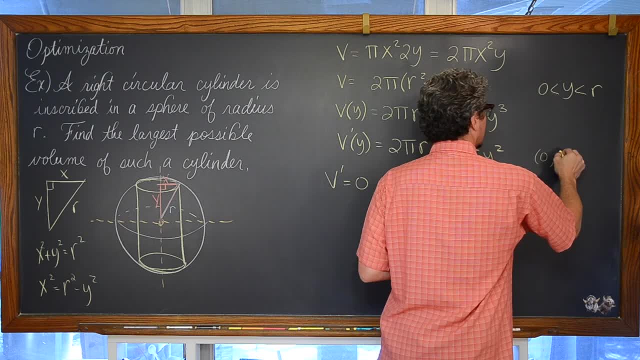 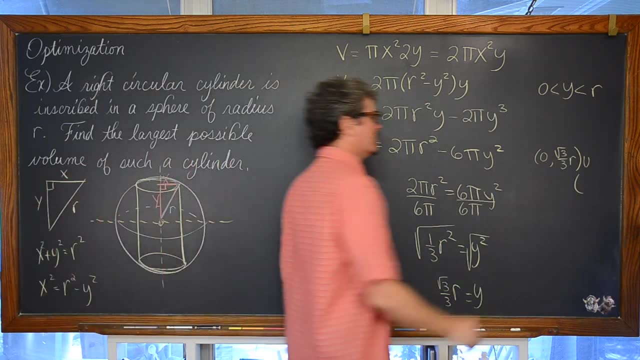 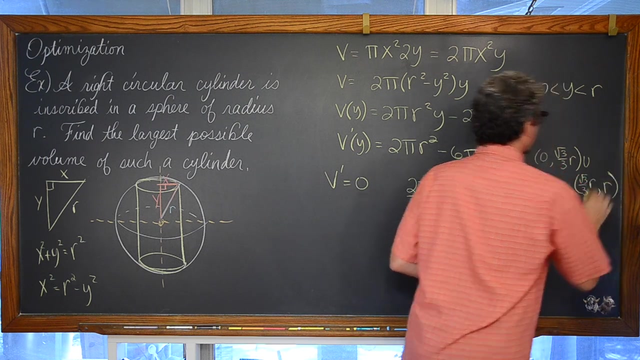 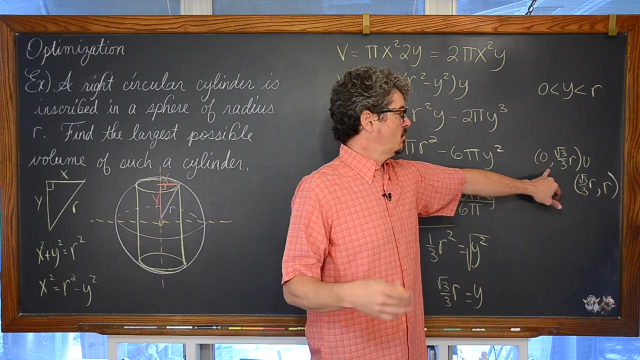 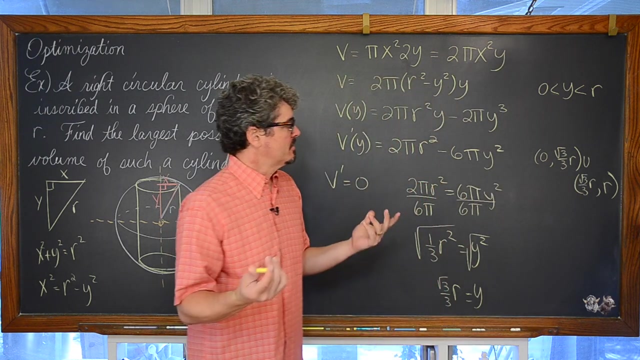 and analyze the interval from 0 to the square root of 3 over 3 r And then analyze the interval from square root of 3 over 3 r to r. So maybe, I don't know, maybe you pick something like 1. fourth, I think that's somewhere between 0 and square root of 3 over 3.. So maybe you 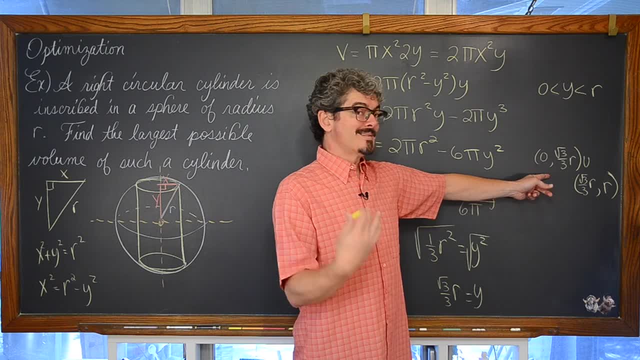 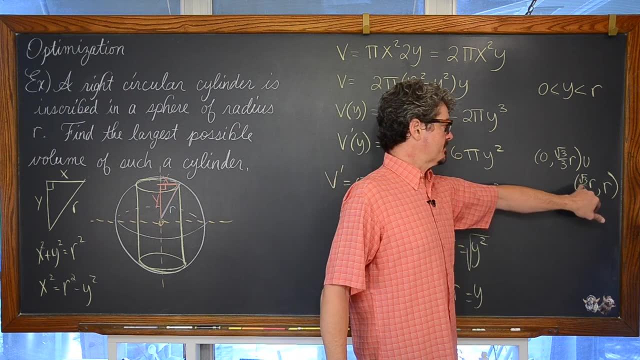 do like a 1 fourth or 1 fifth, or just you know some 1 tenth r and plug it into your first derivative to see if it's positive or negative, And then maybe because obviously square root of 3 over 3 is less than 1, so maybe you 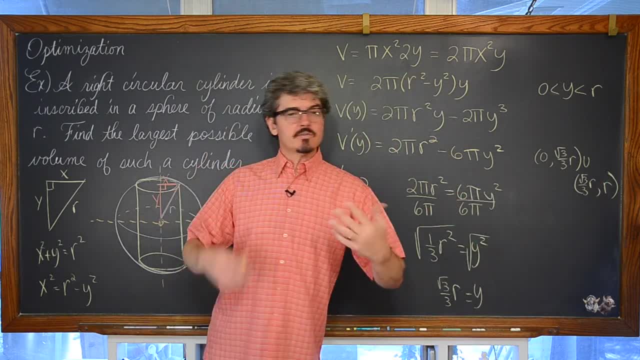 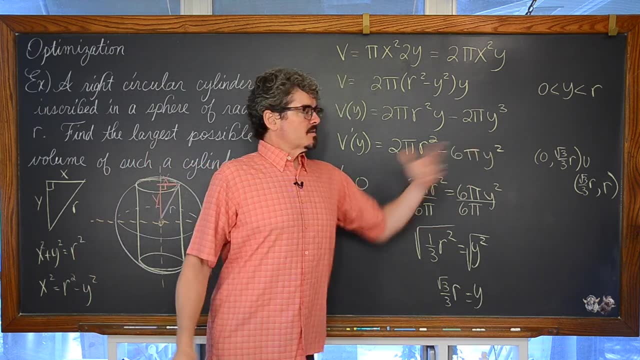 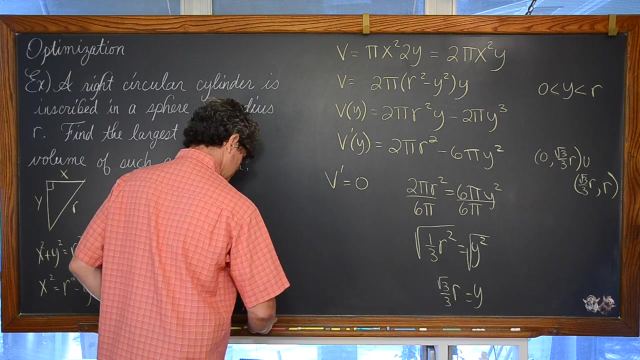 take a 1 r and plug it into your first derivative to see if it's positive or negative and look for that sign change and do that first derivative test. But remember when I said that this is basically just a polynomial. If we look at the second derivative and instead of lookinganalyzing- 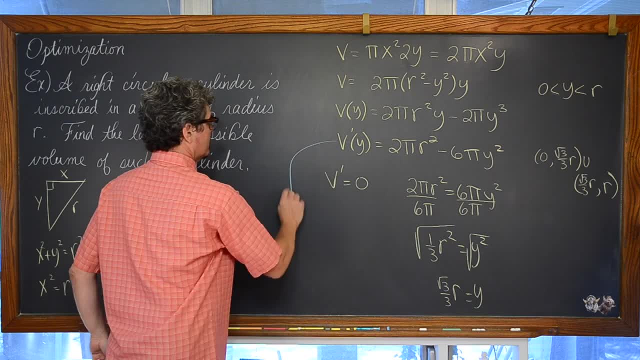 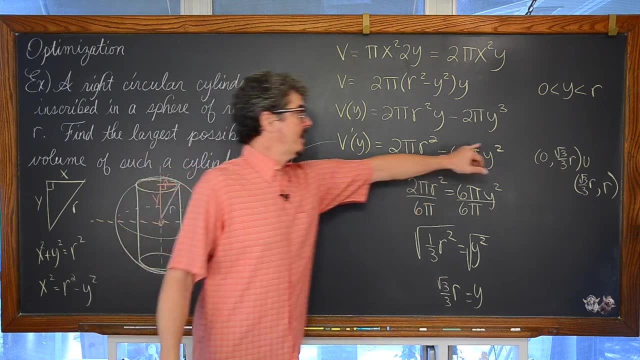 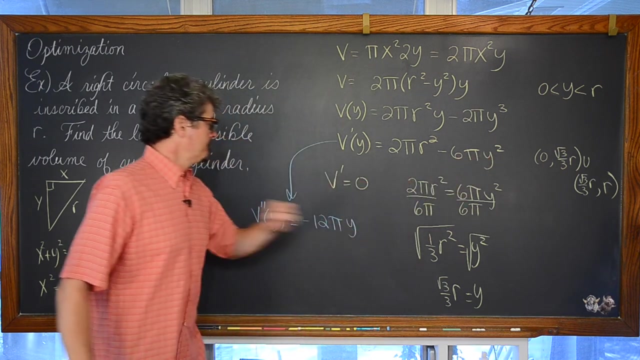 sign changes on the first derivative. take a look at the second derivative and think of the second derivative test. We have v. double prime of y is equal tothis is a constant, so that is 0. And we have negative 6pi times 2, which is negative 12pi y And y is defined to be a positive value. Therefore, 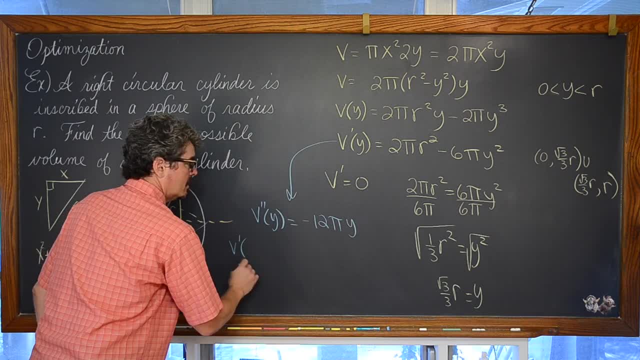 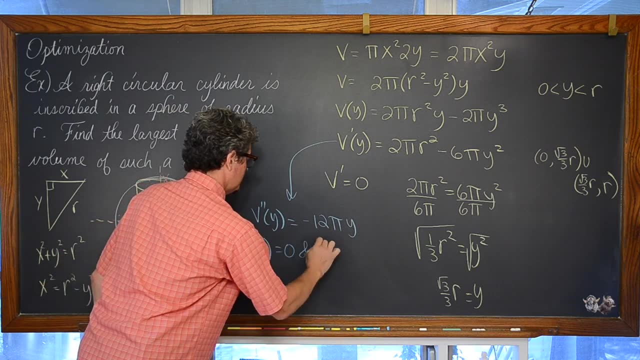 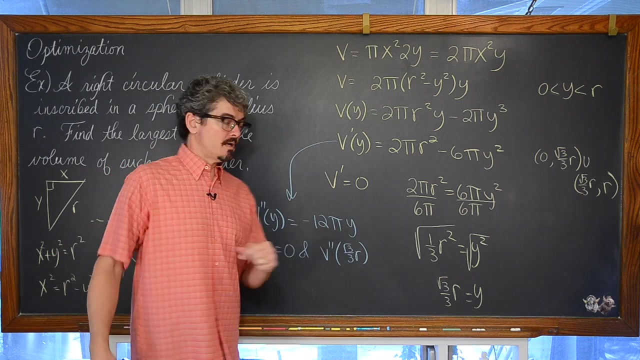 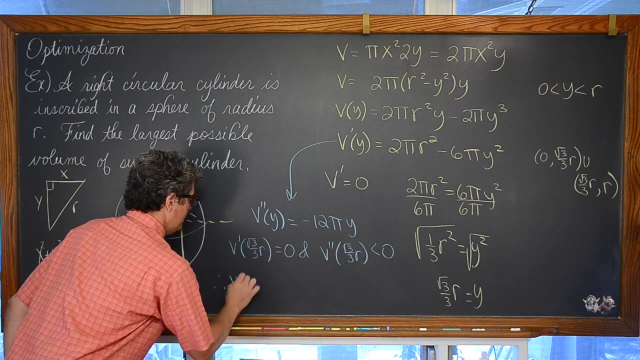 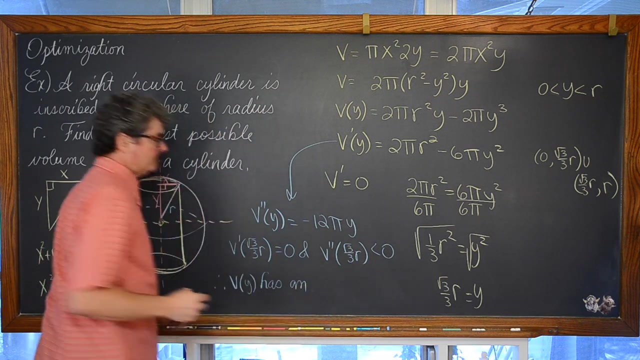 we can say that v prime of square root of 3 over 3 r is equal to 0.. And v double prime of square root of 3 over 3 r is what Negative 12pi times a positive number is negative. Therefore, v of y hasand now for purposes of space, here first and second derivative. 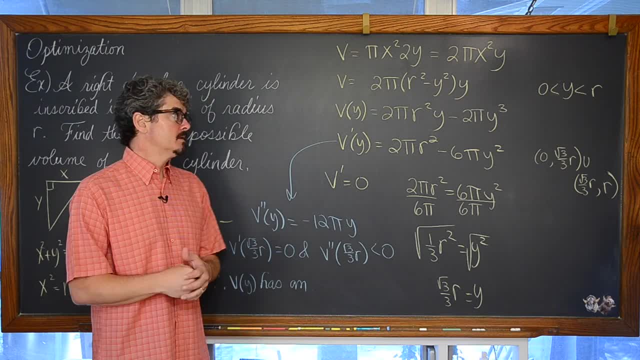 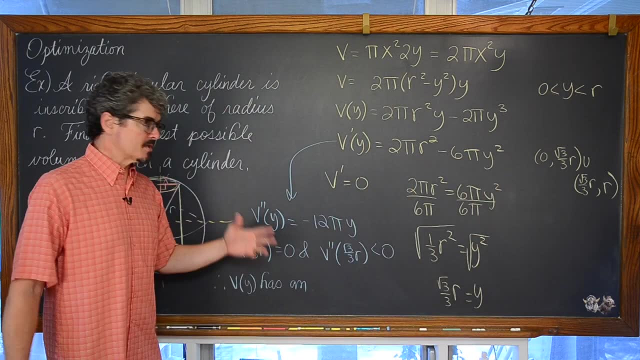 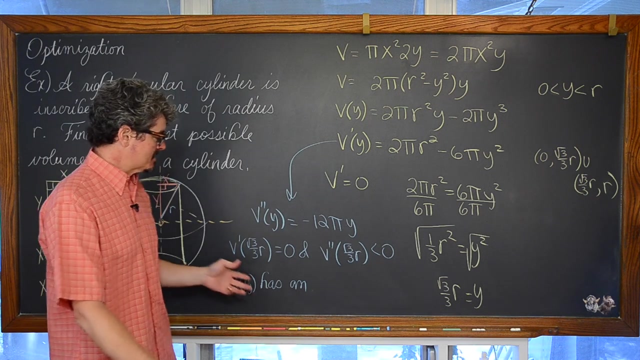 test identify relative extrema. However, this is the only critical value on this open interval and therefore this isn't just a relative extrema, it's actually an absolute extrema. But if you really need to be super specific with your language, you're going to need to add something like: this is the only critical. 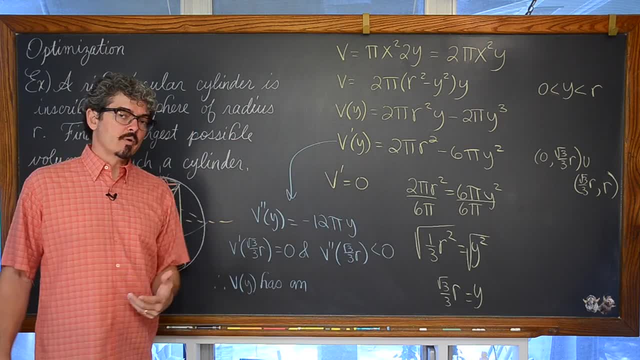 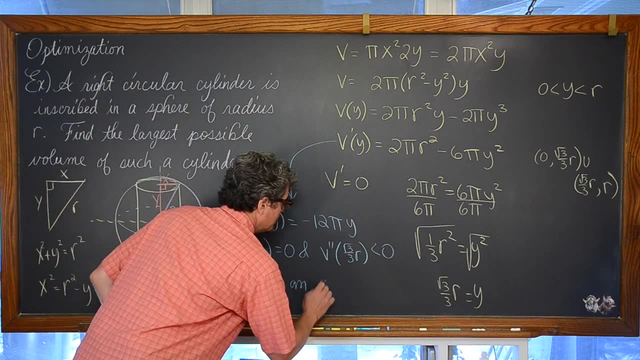 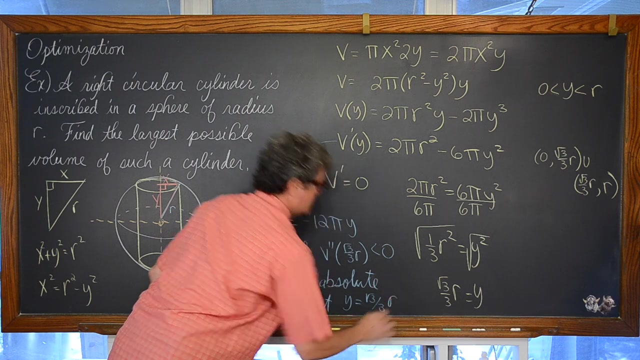 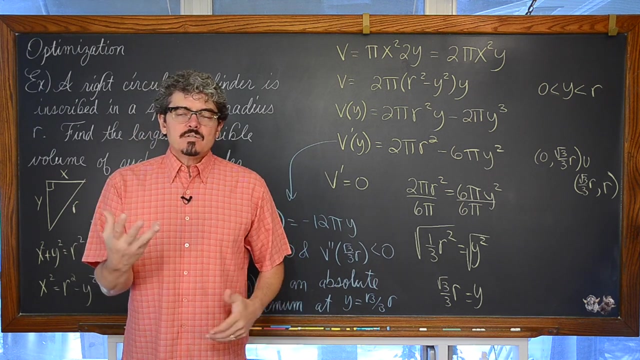 value on this open interval and these conditions are met. Therefore, you have a location for an absolute maximum. I'm going to leave that out because I'm running out of room. So therefore, v of y has an absolute maximum. y is equal to square root of 3 over 3 r. Now we got that validated. The question didn't. 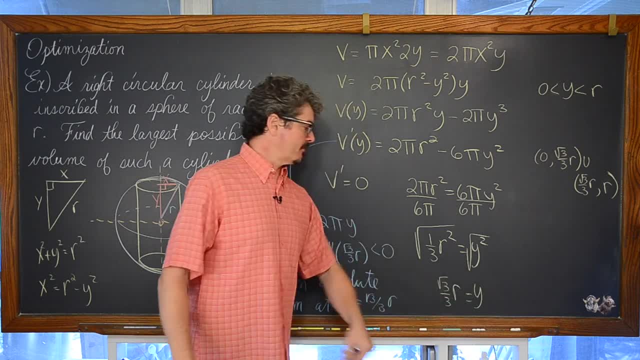 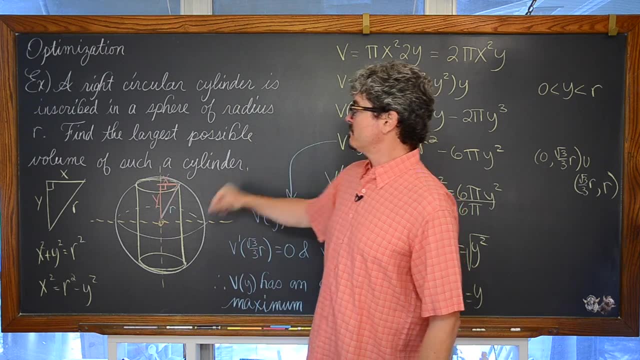 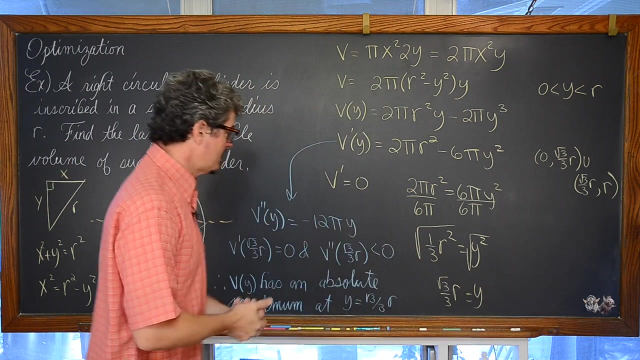 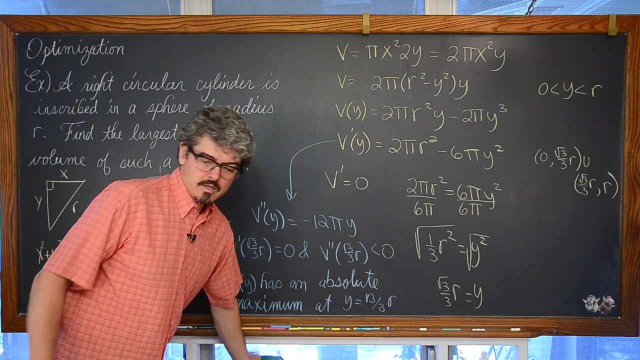 ask for you to find the location, or for what value of y does the cylinder have? its absolute largest possible volume. It asked for the largest possible volume, So now we just have to take this value of y and plug it into our volume function and simplify it. I'm going to try. 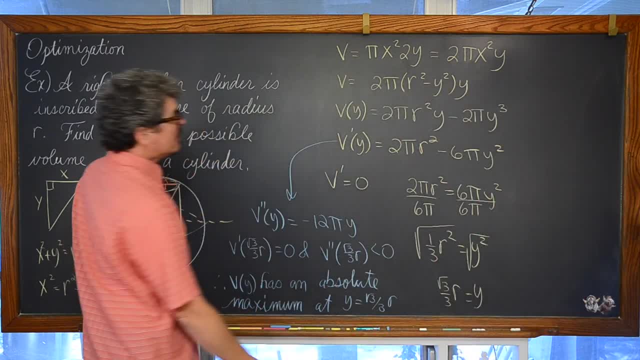 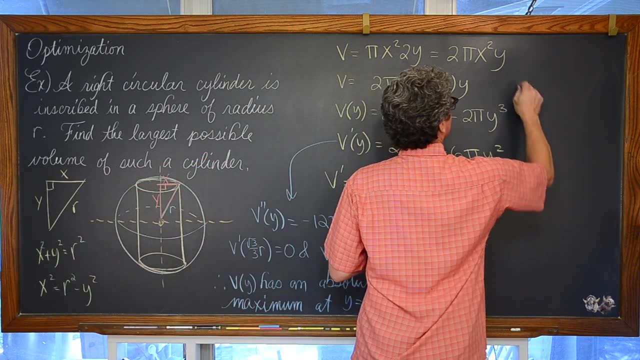 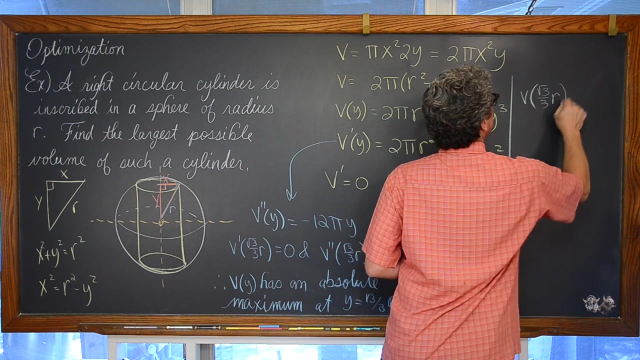 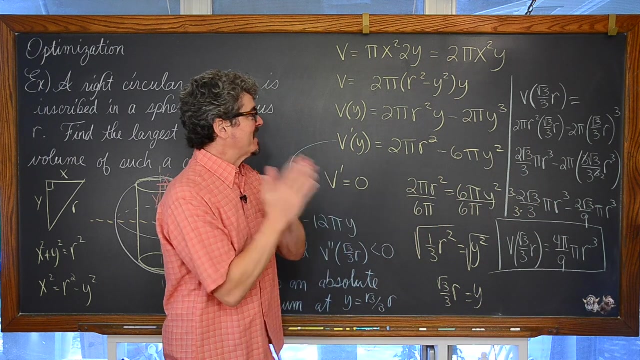 to squeeze this in here, because when I do my videos I like to have it all together for you on one screen. So v of square root of 3 over 3 r is equal to 2pi. I forgot my r and I ran out of time, So let's just finish this up again. We have 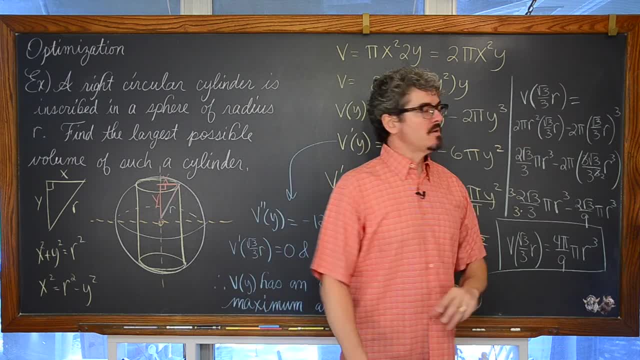 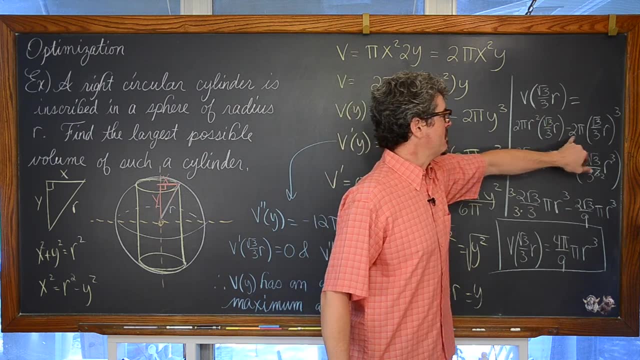 v of square root of 3 over 3 r is equal to when you include the r in your substitution. the second time We have that 2pi r squared times square root of 3 over 3 r, minus 2pi times square root of 3 over 3 r, cubed. Well, of course you know, we just have a little. 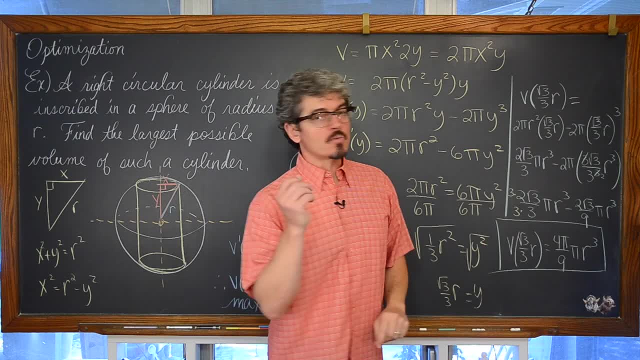 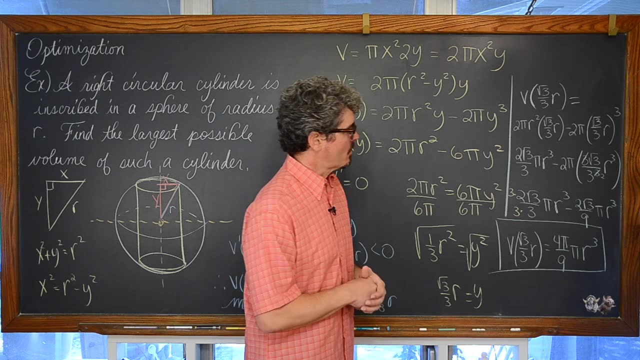 bit of multiplication here in the beginning. Square root of 3 cubed is going to be equal to square root of 3 times square root of 3 is 3 times that additional 1 left of square root of 3.. Our denominator has in it a 3 cubed, but of course 3 to the first divided by 3. 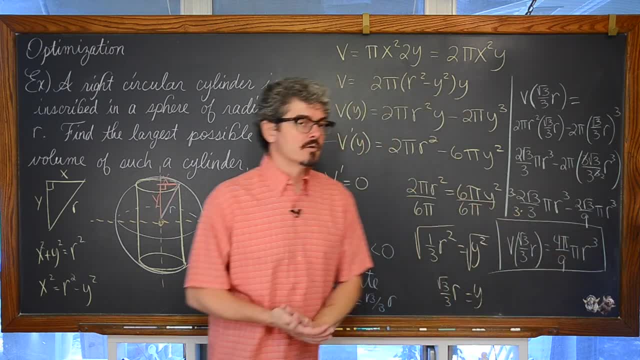 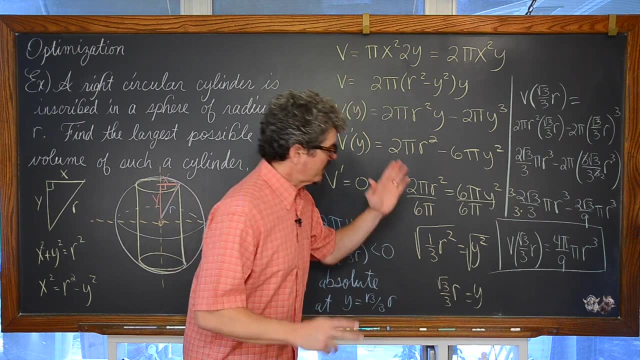 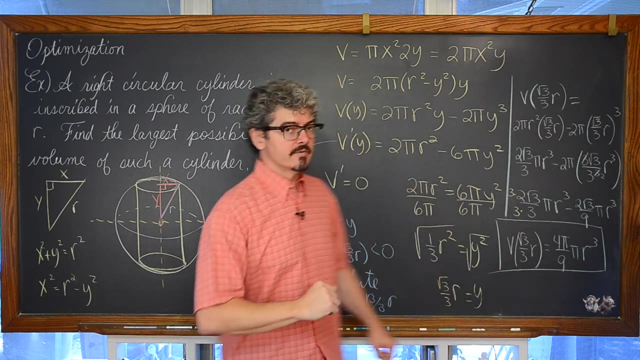 cubed is 1 over 3 squared, giving us a denominator of 9.. In finding a common denominator with our first fraction, by multiplying the numerator and denominator by 3, we have a final answer of which is the maximum possible volume of such cylinder which is inscribed inside of. 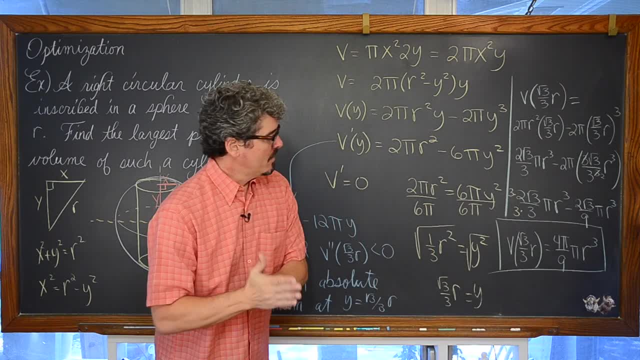 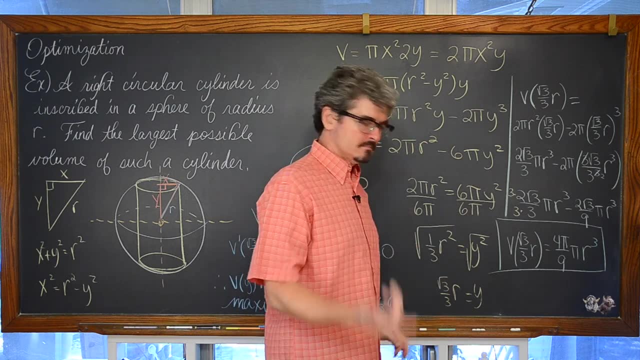 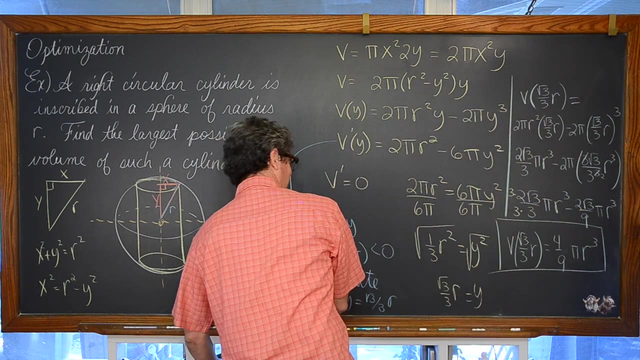 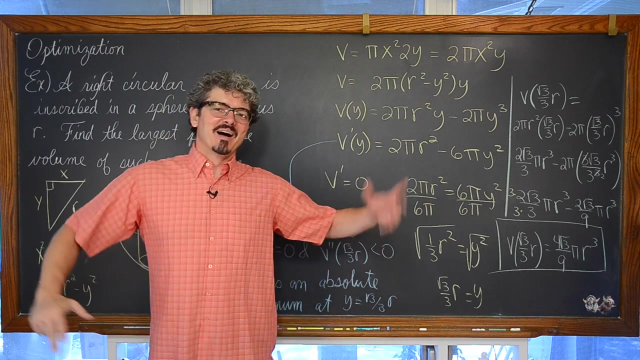 a sphere with radius r V of square root of 3 over 3r is equal to 4pi over 9pi. Let's try that again: 4 square root of 3 over 9pi r cubed. I am Mr Tarrou BAM. Go Do Your Homework. 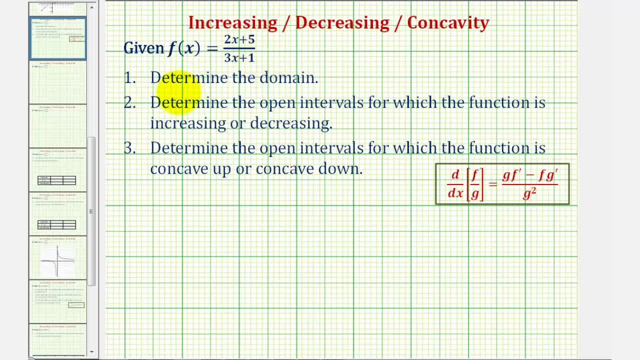 Here we're given a rational function, and then number one asks to find the domain. Number two asks to determine the open intervals for which the function is increasing or decreasing. And then, step three, find the open intervals where the function is concave up or concave down. 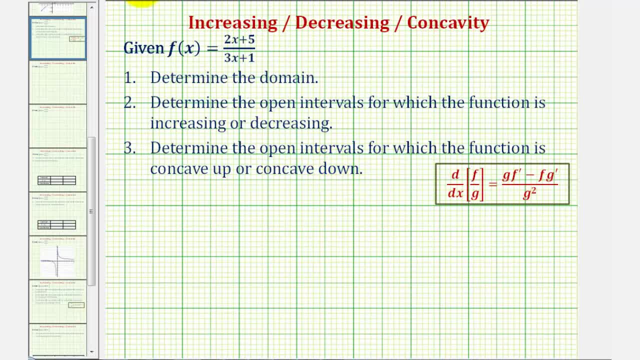 Let's begin by determining the domain of the given function. When working with rational functions, we must exclude values of x where we'd have division by zero or where the denominator would be equal to zero. So for number one to find the domain, we'll determine which values of x we must exclude from. 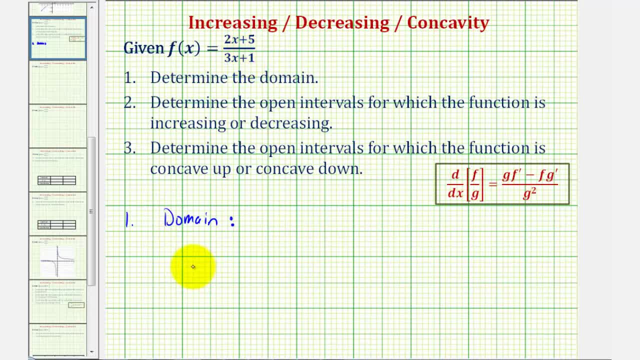 the domain by setting the denominator equal to zero. So if we set three x plus one equal to zero and solve we'd subtract one on both sides, So we'd have three x equals negative one divided by positive three. So x equals negative. one-third would make the denominator equal to zero. 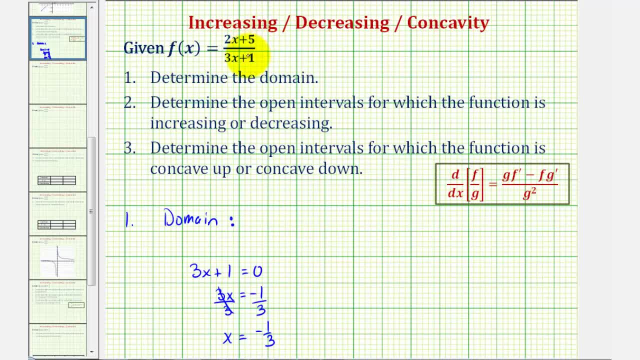 meaning we'd have division by zero and therefore the function would be undivided. So the domain would be all real numbers except negative one-third. So using interval notation we can say the open interval from a negative infinity to negative one-third union, the open interval from negative one-third to positive infinity. 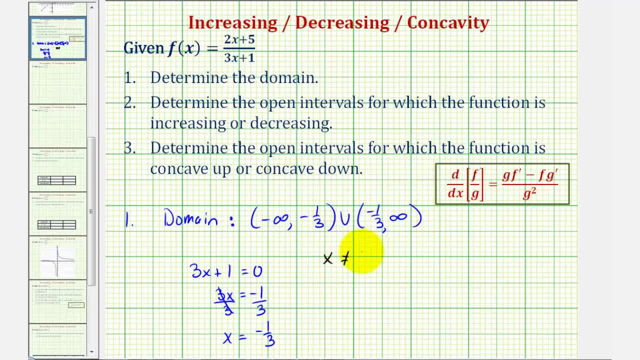 Some textbooks also just say x can't equal negative one-third. or we could say: all real numbers except x equals negative one-third. So there are several ways to express the domain And now determine the intervals for which the function is increasing or decreasing. 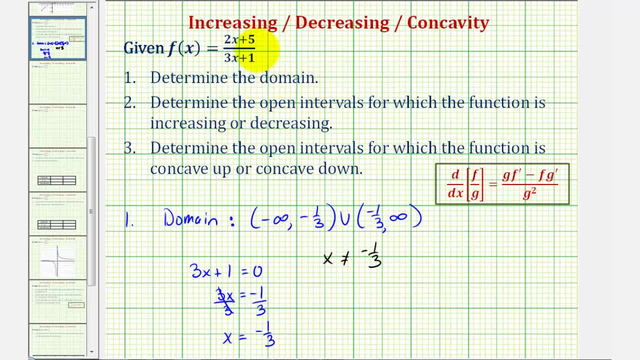 To do this, we'll first find the critical numbers of the given function, which would be where the first derivative is equal to zero or undefined. Once we find the critical numbers, we'll divide the domain of the function into intervals and test the sign of the.